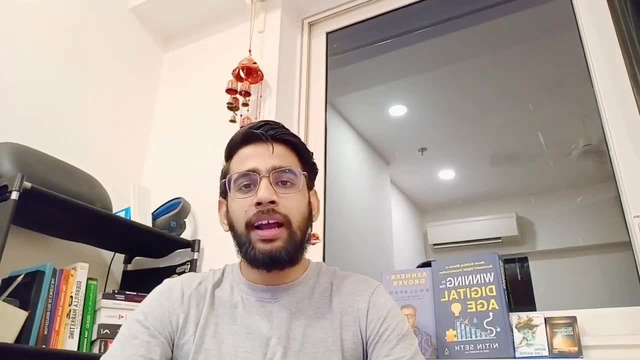 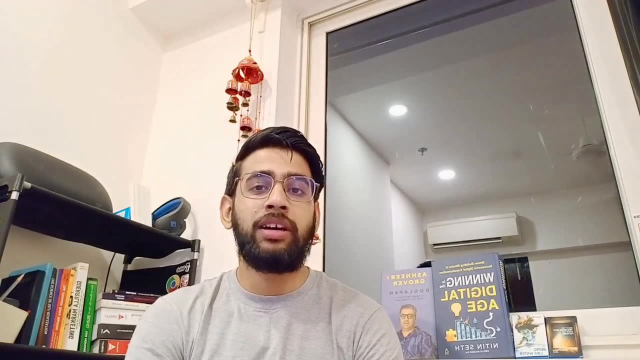 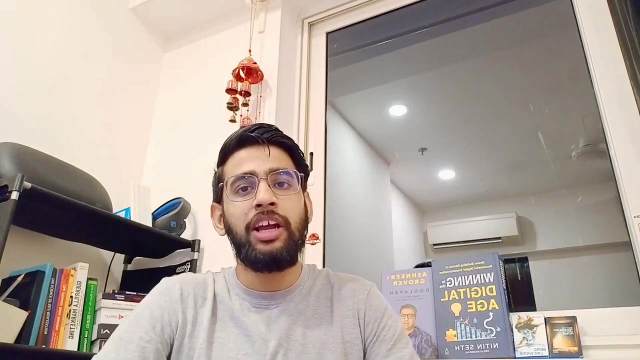 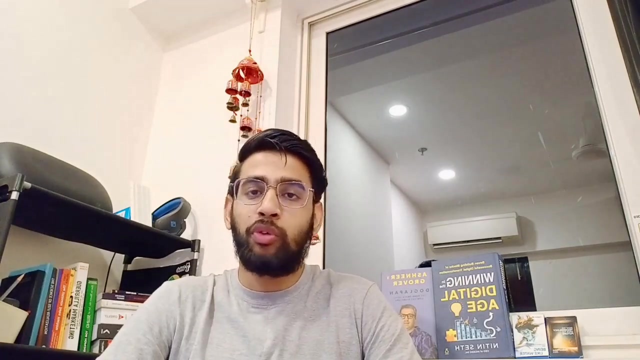 released the paper and the weights are still not available, but they are smaller in size when we see the other competing models for code and they are 1.3 billion parameters and also they have released Phi1 small which I reckon is 350 million. So they have basically considered a different technique, a novel training process basically to train this model and come up with you know something which can compete with already existing large language models for code. Because you know we have seen over a period of time that putting more parameters, the more layers into this language model that has been trained recently. This has been the basically the scaling 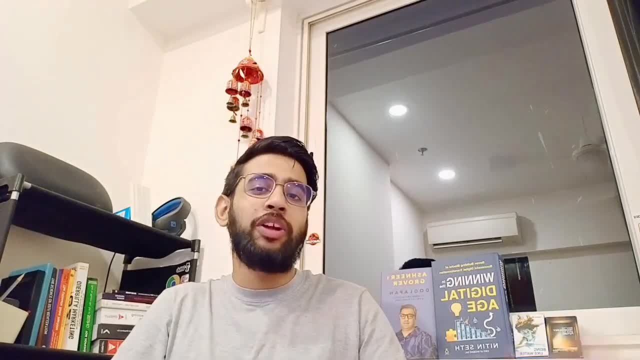 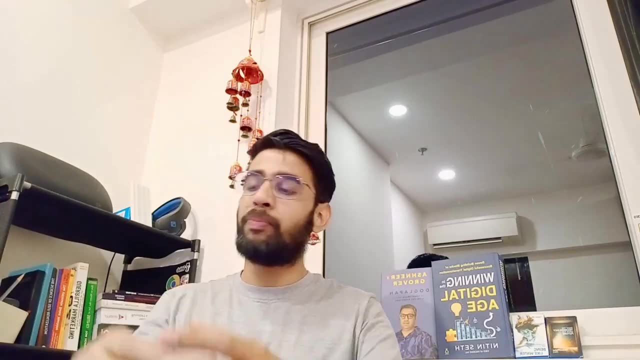 law I will say. That people say okay put more parameters and your large language model will be better. But you know what Phi1 has you know the people, the researchers behind Phi1, they have 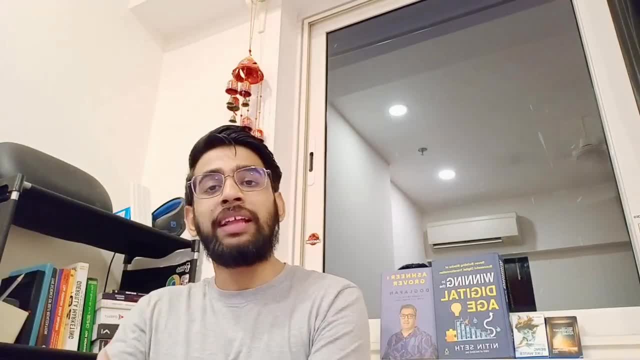 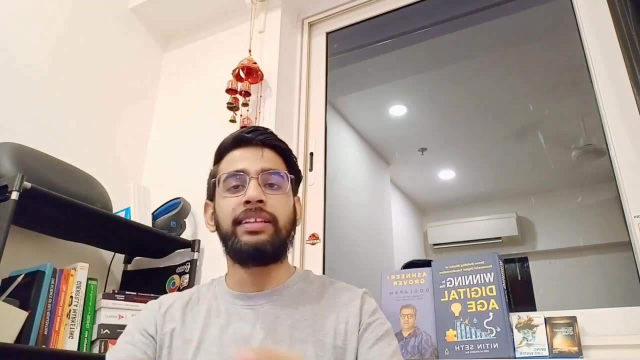 basically done a lot of research on this. They have done a lot of research on this. They have basically done a lot of research on this. They have done a lot of research on this. They have basically taken a other route there and they have focused more on the better data quality or a high quality of data you know a better data model while training these you know large language models. 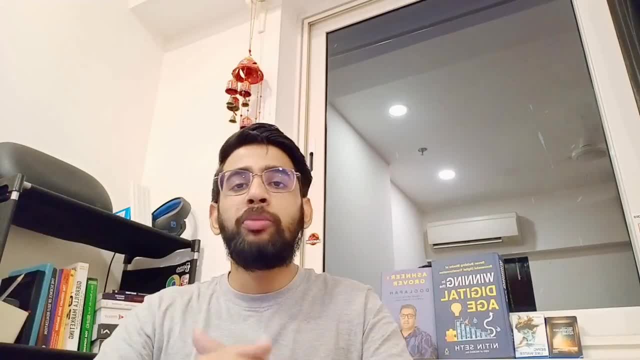 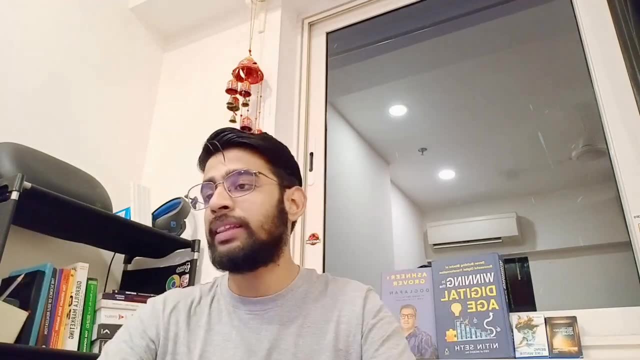 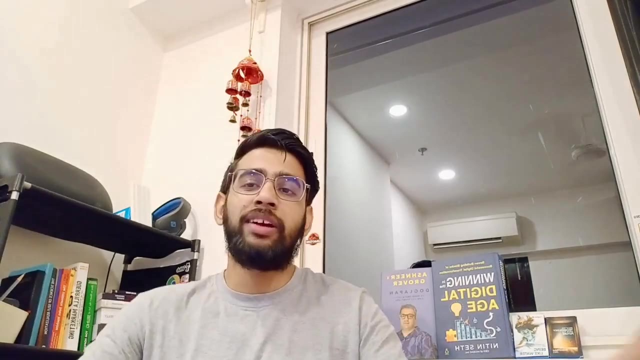 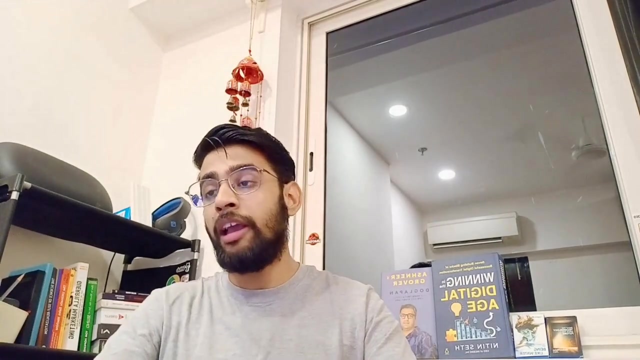 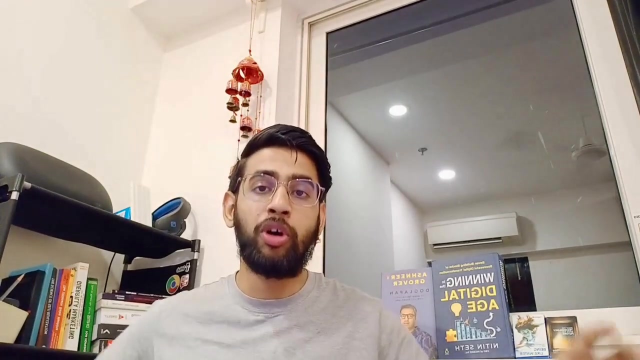 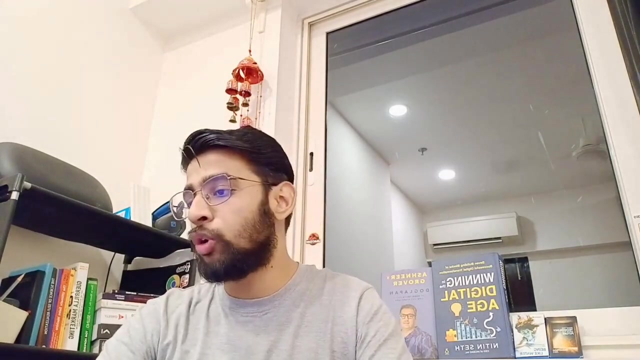 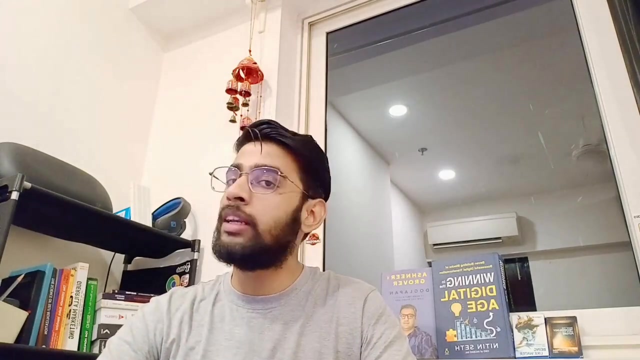 They have a very novel approach and you know mainly in this video because I have done a pretty good study on this research paper and I have come up with my perspective that I will explain basically and it will be pretty theoretical video guys. Because you know the weights are not available for this. I don't know if that is going to be an open source model and let me know if you have any information on that one the availability of this model because currently it's not available and there has been some talk in the community. They are discussing that this model will basically will be available on Microsoft Azure. So if you have any information related to it please let me know in the comment box. But this video you know it's going to be completely theoretical. I'm going to explain. 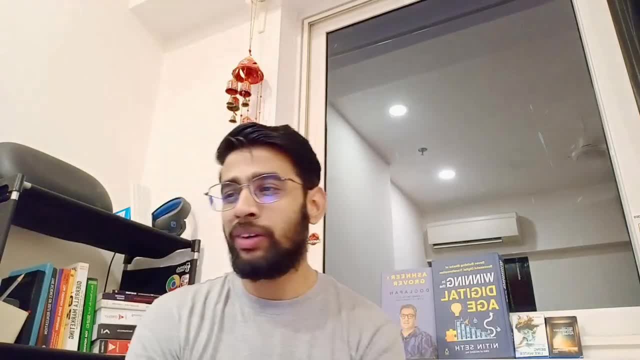 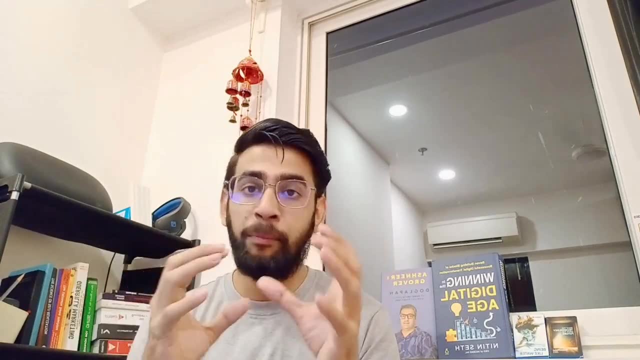 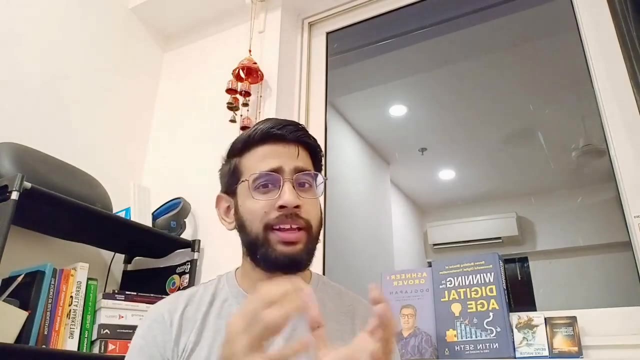 You know that how they have trained this model, what were their data strategy to come up with this high-quality data and how they have created this sort of data basically and what kind of embeddings have been used on top of it, what kind of classifier has been used. So if you are not a theoretical savvy person, I will request you not to watch this video because this video we are going to talk 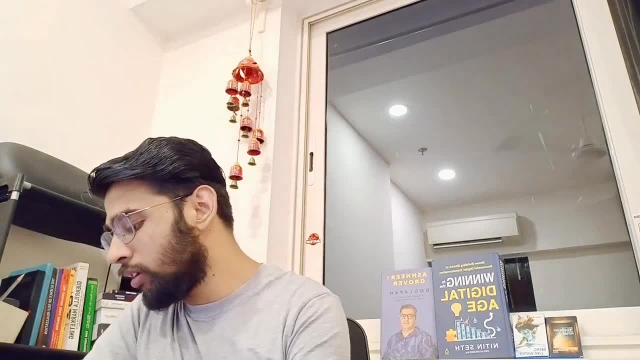 theoretical, we are going to use our you know the screencast and make all the video. It will be secreted and not being created. So if you have any questions please let them know in the comment box. 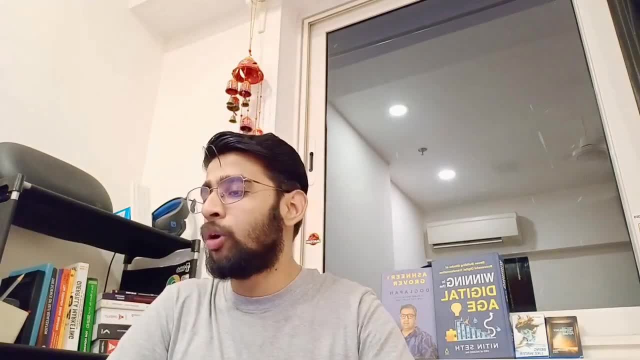 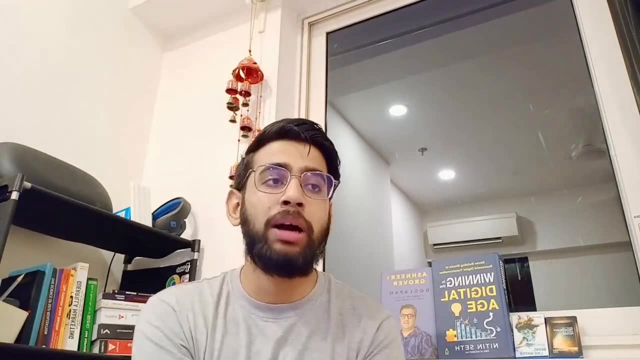 and all those things that we'll explain it on a board and i hope it will help you understand that how you can also come up with your research in these areas because i myself you know i'm 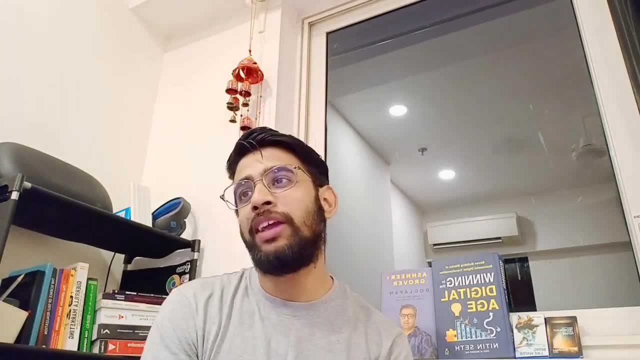 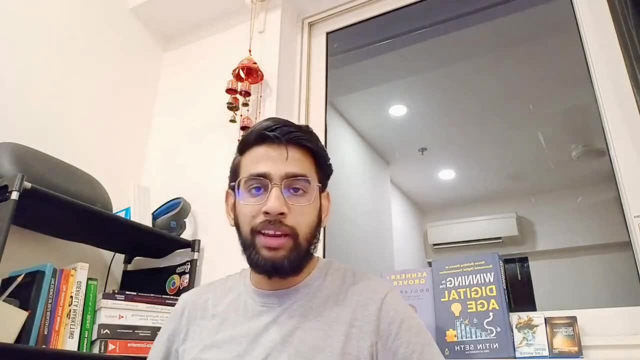 associated with some research group we have we are trying to do something in this field we are also you know in the process of experimentation on a few things that i will explain you in in 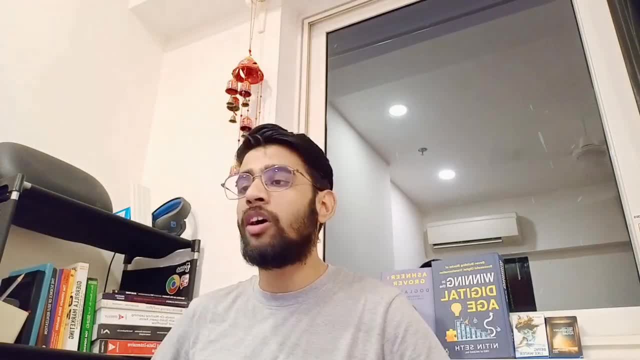 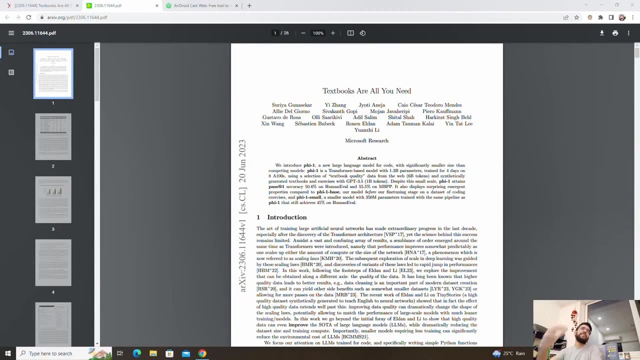 the upcoming video okay so in this video let's start on this five one so the paper name is textbooks are all you need like in 2015 or something that i think i forgot the year when the transformer was you know was released by google i think the paper was attention is all 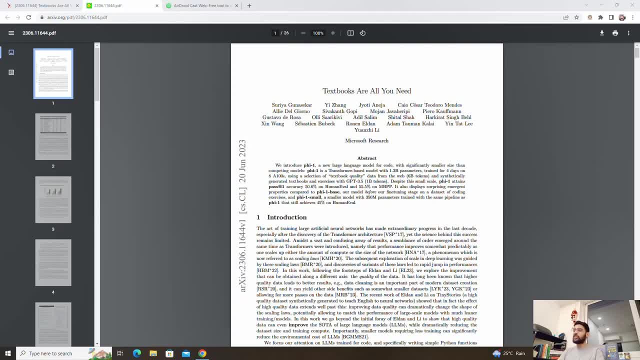 you need okay so i really like the name as well so let's jump in so if you see here you know i am on this research paper textbooks are all you need the researchers by microsoft research 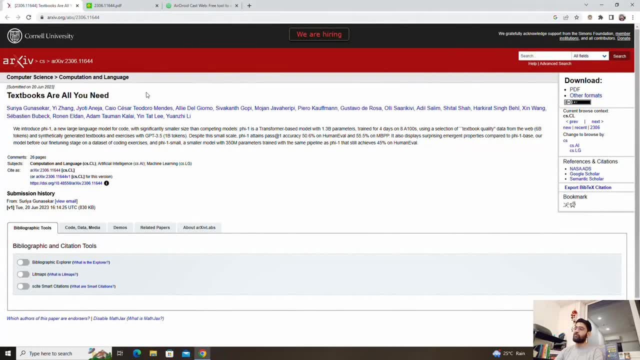 and here you also have a level here on you can find it over here the pdf you can look have a look at it 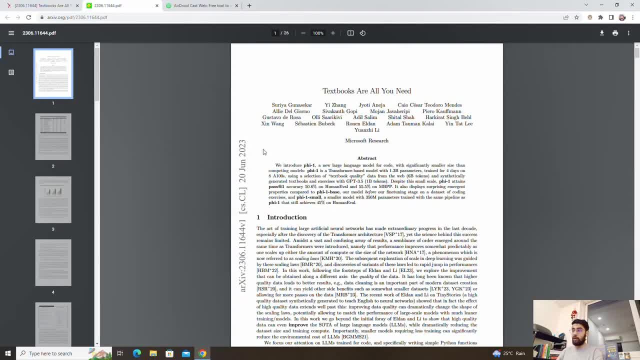 and if you read they say we introduce five one uh new language large language model you know for code it's more inside that i already told you 1.3 blah blah blah and the human evil and mbpp has been the again the benchmark for evaluation there when you see it on that so i let me show you guys okay 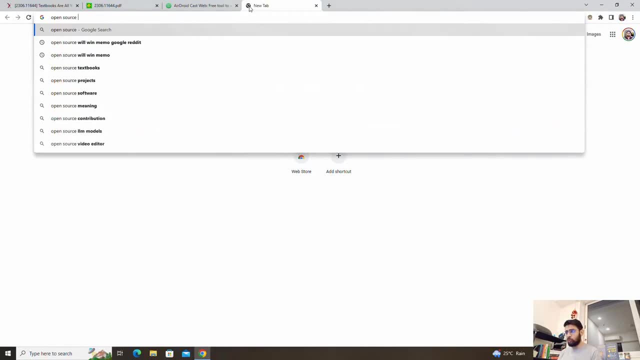 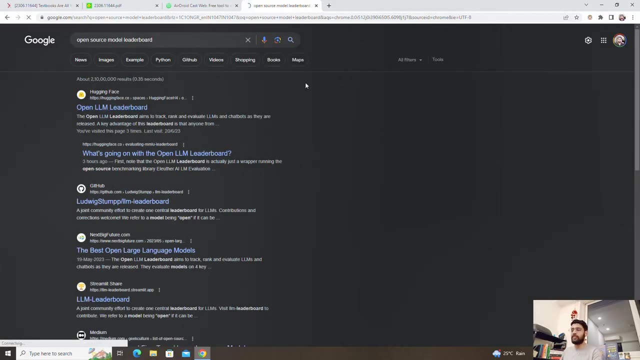 how you can do it yourself so there is one open source model leaderboard by hugging phase okay leaderboard which is again been you know it's easier for tracking this 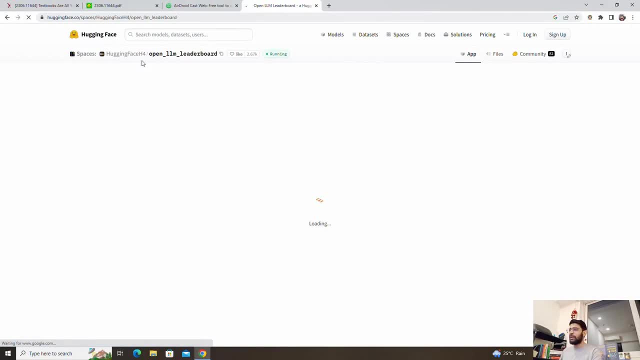 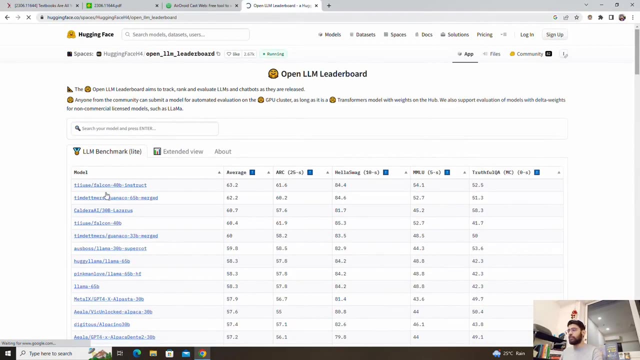 language models if you see here see it over here this is by hugging phase h4 open llm leaderboard you know falcon came from uh some from arabian countries if you see here the falcon for tv 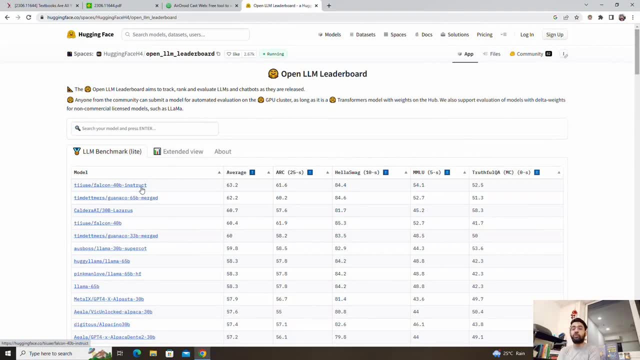 they claim that they are you know they are that their open source model is the best one based on this you know uh that evaluation benchmark that we have on you know human eval and you know mbpp etc for example you can see all the listed language model the large language model the 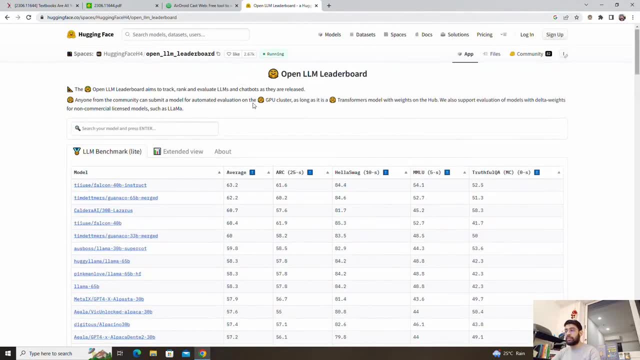 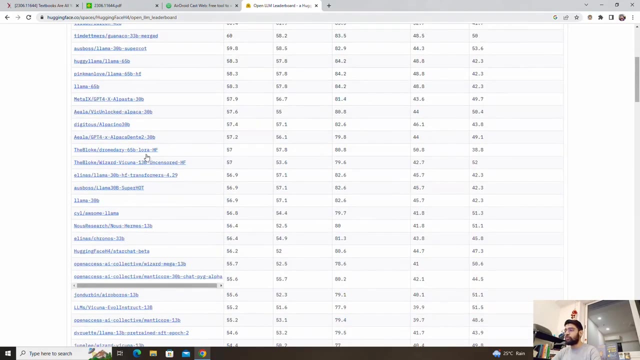 open source language model this is only for open source llm it's a leaderboard so you can find it out that falcon for tv is leading okay on you know truthful qa mmlu you know and all this uh that that this kind of tracks it easier to track so if you want to use of one of these models maybe you can 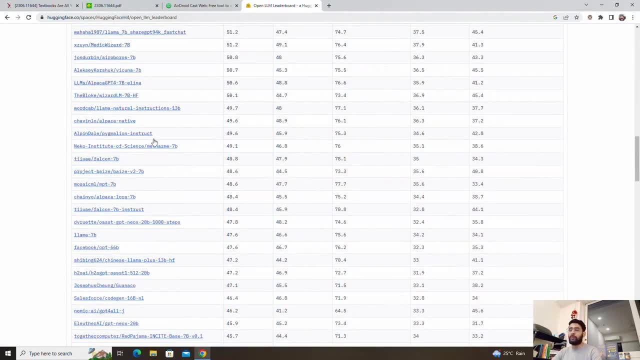 just click on that and it will take you to the you know repositories and space as well so maybe you can have a look at it okay and 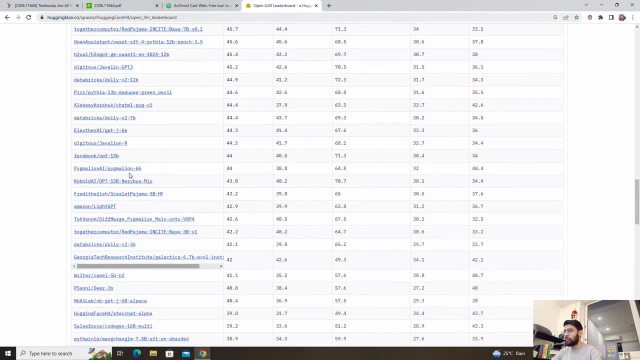 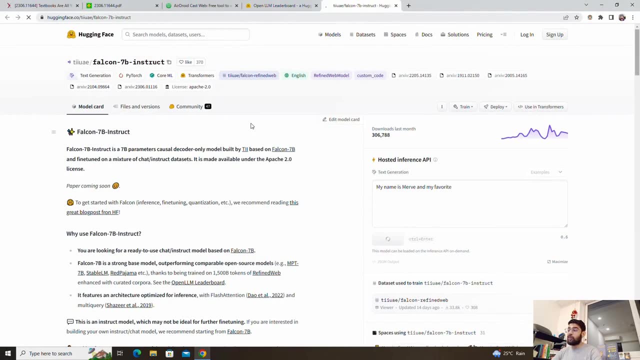 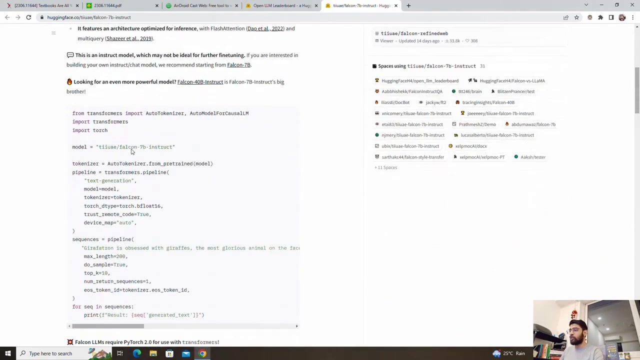 for example you know if you want to have a look at um falcon 7b instruct that might run on a consumer gpu as well and if you can run it on your if you don't have a high compute infrastructure maybe you will you will fancy running or influencing the 7b model so you can look at it here they they have given you the code base etc text generation the pipeline over there and then 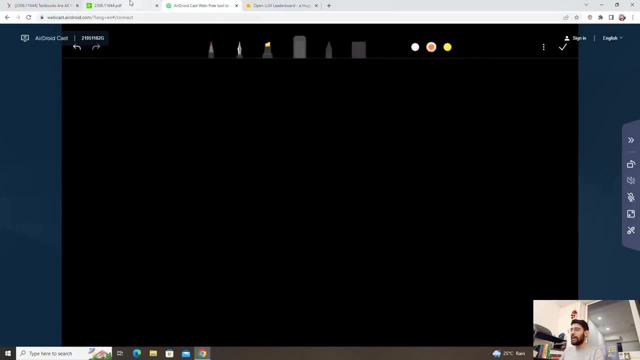 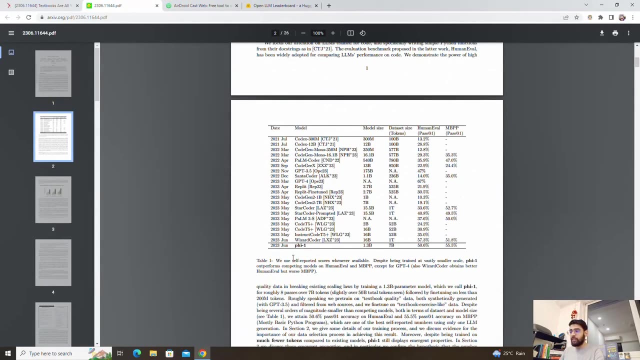 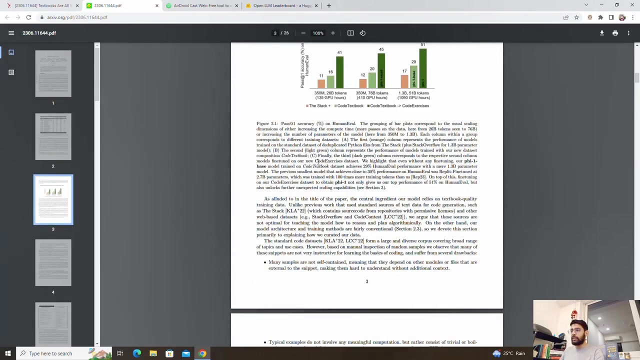 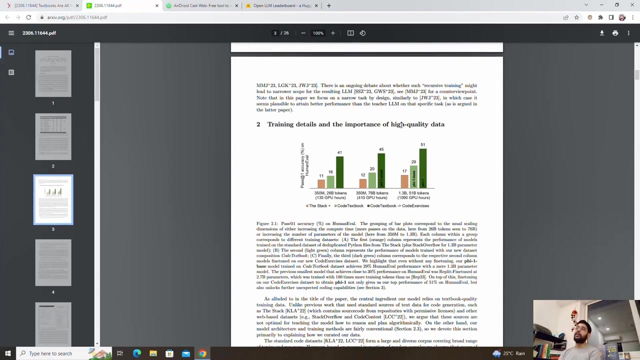 you can also have a look at it now let's come back on this textbooks are all you need here is a research paper and you can look at it that how this has been you know that basically courtyard has been used i will explain that about the embeddings as well and the embeddings part and you can see training details and the importance of high quality data because i do believe you know i echo the thoughts here that you know we have to rely on high quality data rather than putting just you know putting more travel parameters 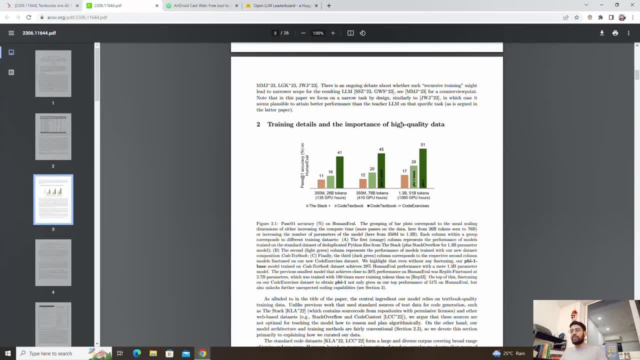 have to considering those factor will not take us anywhere I believe because you know when it reaches that stage where you don't have that computation power in your data center what will you do at that stage how will you get all 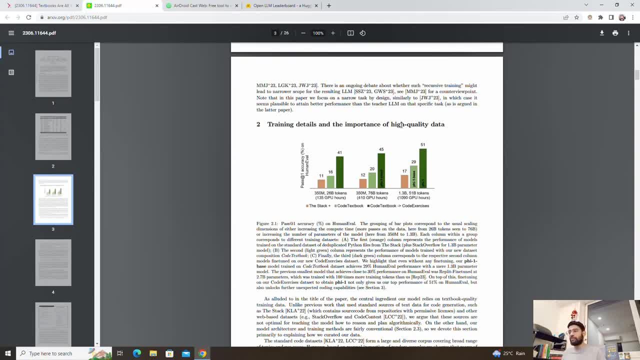 this energy I don't know if you heard about bloom by hugging face which was trained by capturing the energy from nuclear reactor you know I don't know if 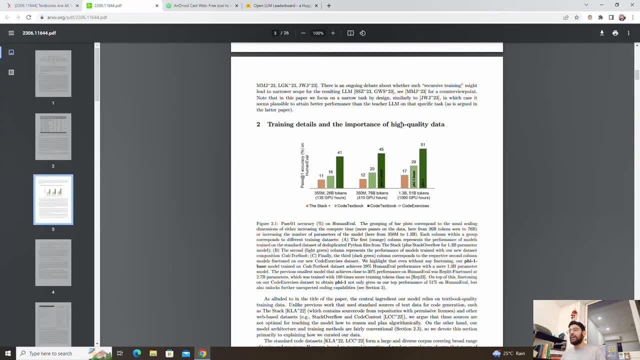 that's true but you know there were some discussions in the reddit community on on bloom how it was trained so I think we have to focus on some other 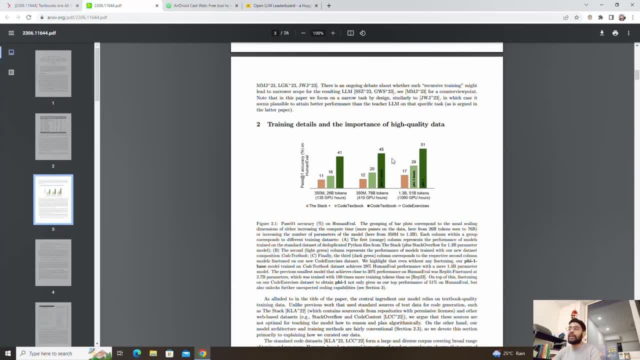 approaches some different approach of getting more accuracy and becoming better when we talk about this LLM based responses and that's how five one might 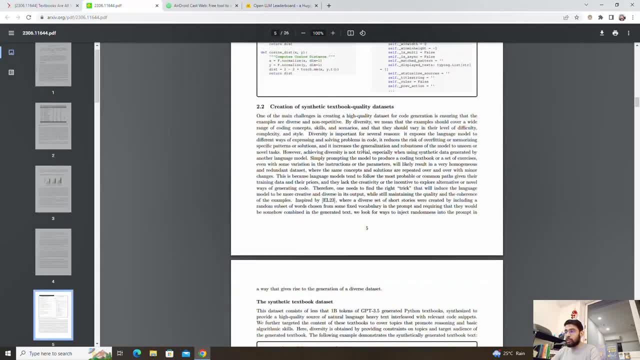 be the you know a starting point here and you can see that educational value they are talking about education that I'll explain that what it means very 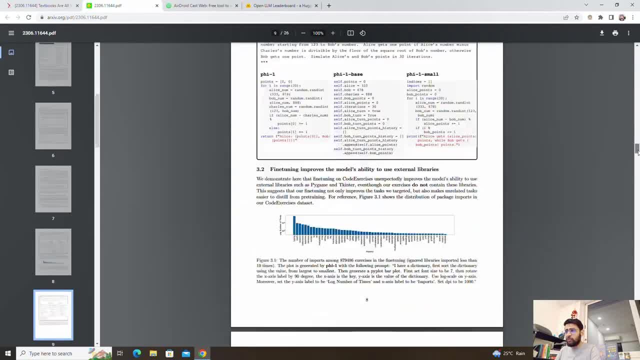 quickly now if you see this is the research paper you can find it the 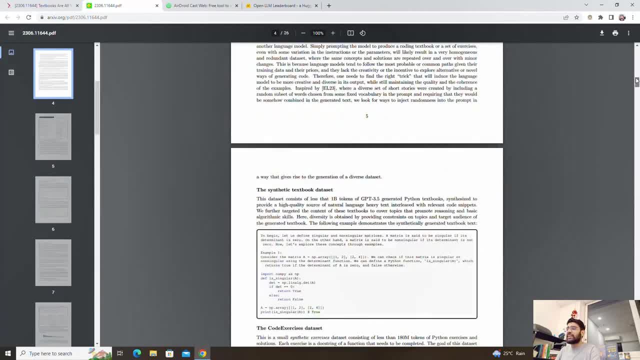 conclusion and then there's a embedding and so let's start let's understand a bit I'll explain what I am from my findings okay the finding that I have you 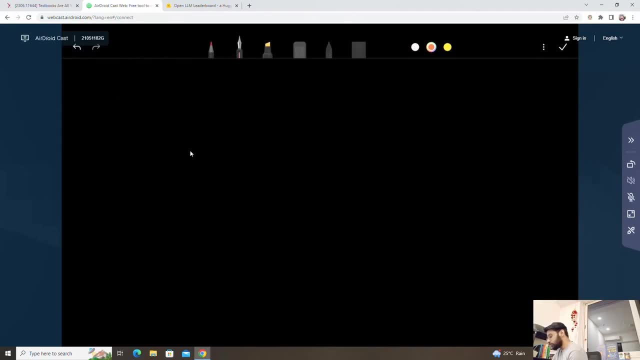 know it will be little theoretical as I said so I hope it's visible here yes so 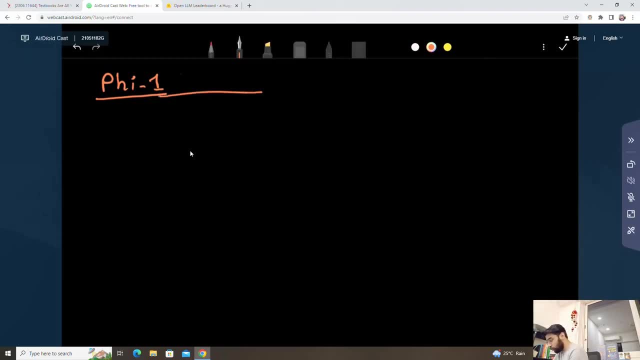 five one let me write it so maybe this will also help you as you know as a note five one by Microsoft because no when I was 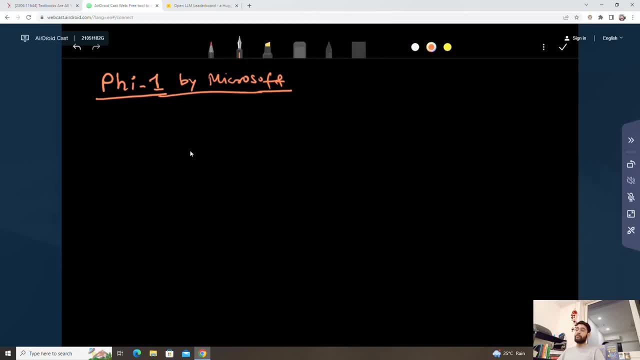 doing my study on this research paper I really loved it okay so I have made a note out of it guys no but I will I'll not cover the entire nodes because it will be too big of a video to you know create but just a high level overview that what are the techniques how have they come up with this model guys the 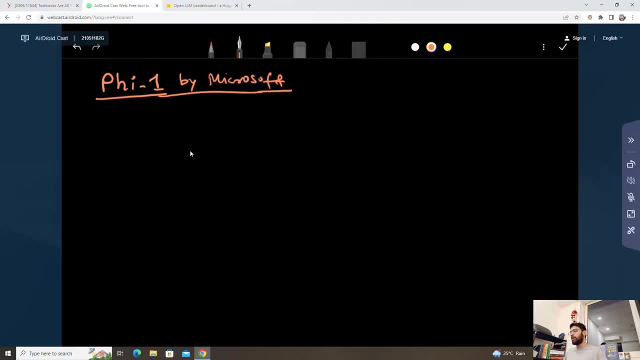 architecture the data strategy everything become very high level so five one by Microsoft of Microsoft again and Microsoft and llama it's like a water 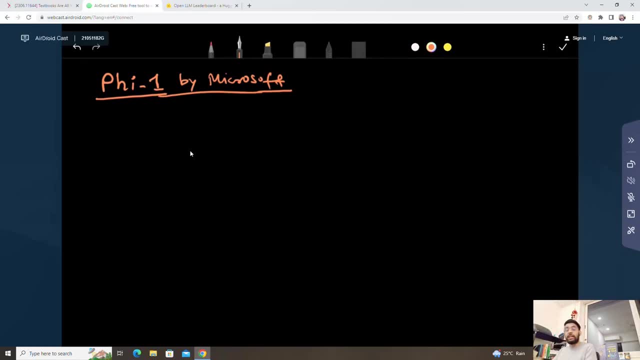 now okay on the language models so you know it's not llama but it's this meta meta A and Microsoft and lama it's like a war now okay on the language models sorry not lama but it's this meta meta A and Microsoft and llama it's like a war now okay on the language models sorry not lama but it's this meta meta A and So, PHY1 by Microsoft, it's a very novel training process that they follow and we will discuss about this training process in details. 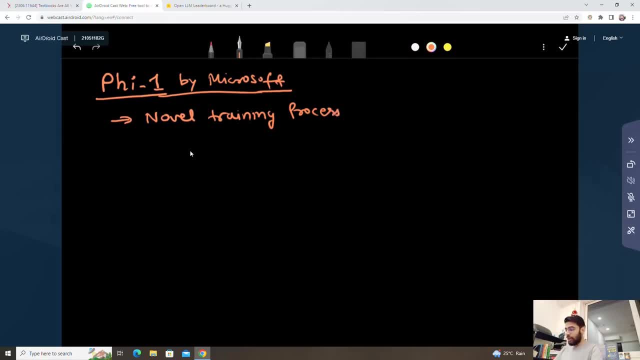 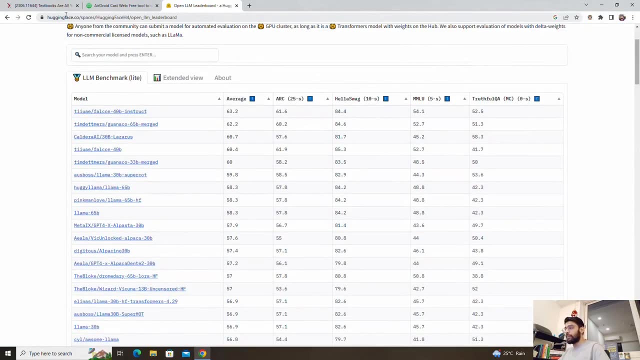 What are the steps that we have in this training process? And if I just give you this, we are talking about human eval, if you will, you can also find it over in a hugging face as well. 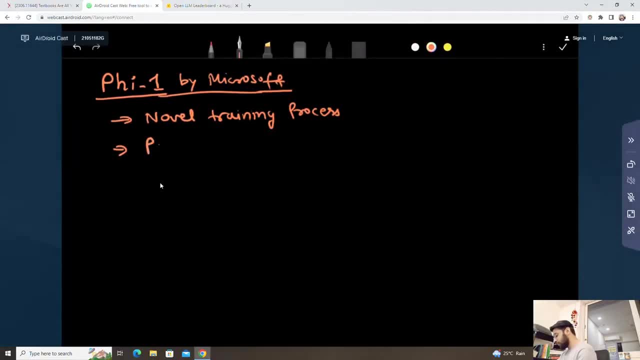 So, the passing rate for this model, the passing rate is of more than 50%, it's around 50.6% on human eval. That's what we use currently in open source community at least to benchmark this language model, so the large language models in general. 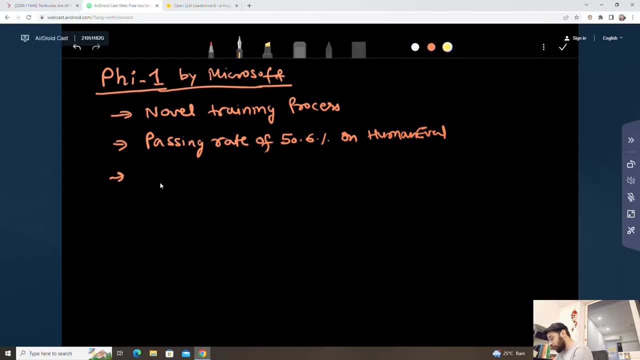 But the problem right now with PHY1 is... And I was expecting, but it seems like this might not be an open source model, I might be wrong there, but the weights are not available. 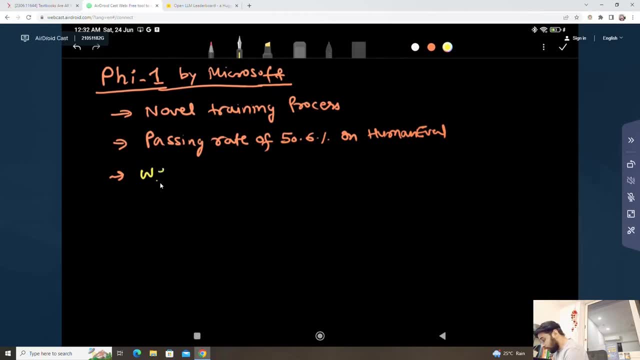 So, if you see, these weights are not available, so weights are not available. That's the biggest, I'll say the challenge right now, because I wanted to, and I assumed 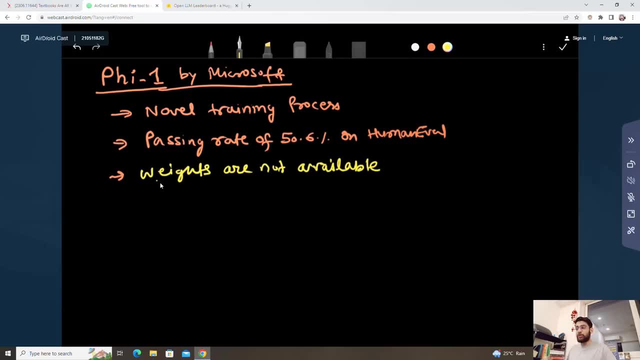 that you would also love to... Basically, at least use this model to see how can we fine tune on our data or maybe on our whatever code basis that we have, basically. 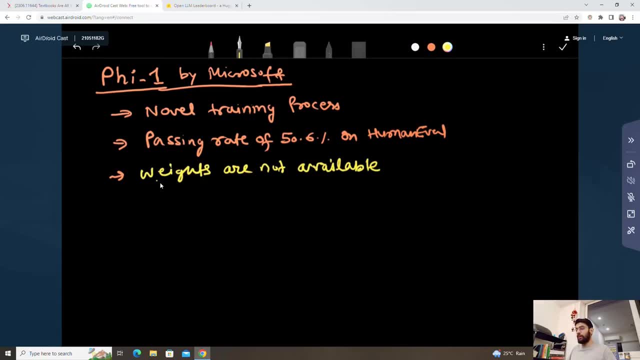 So this is a question that weights are not available and what should we do now, but we'll see that. 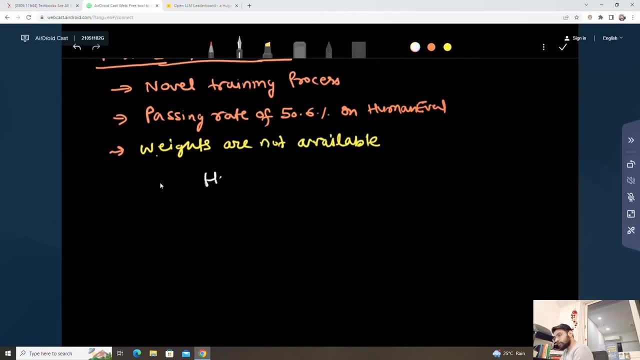 But here is the thing, so high quality data of the focus, the complete focus is on high quality data when you talk about PHY1, and this basically can also change the shape of 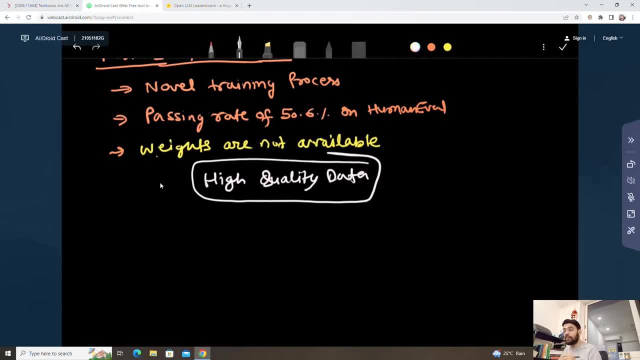 scaling laws, because you're talking about scaling with the putting more layers and we're calling about the trainable parameters, I have 40B, 60B, 70B models, so this basically can change. 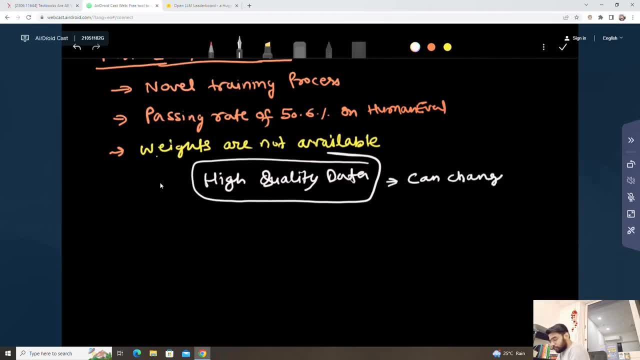 So this can change the shape of scaling laws. 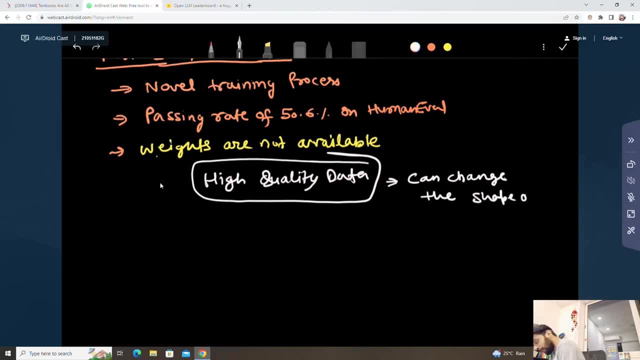 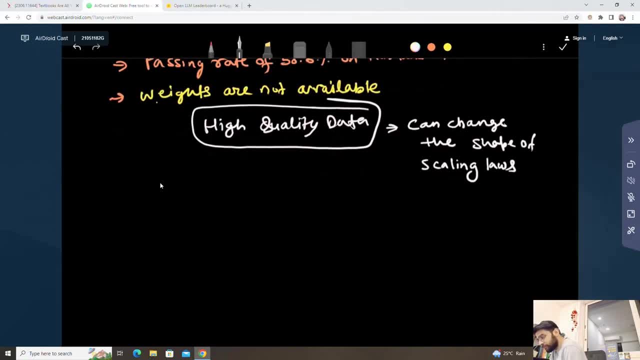 Okay. Okay. Okay. Okay. 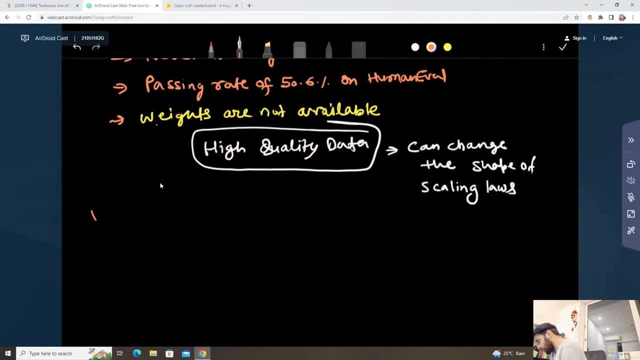 But now how... What are the training extending and how have they trained it? Okay. If it's a question. 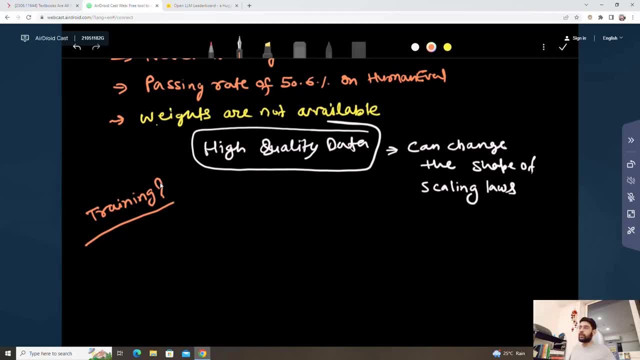 So on the training part available, what are the steps, what are the strategy behind about this training process when you talk about PHY1, let's start with the data. 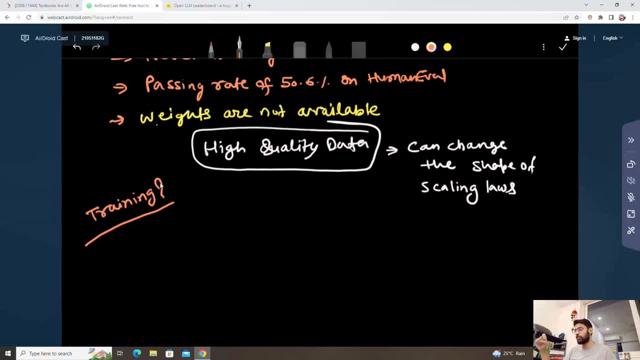 We have to directly jump into the modeling part because it really plays a role here. So they basically have trained on a new dataset. Okay. 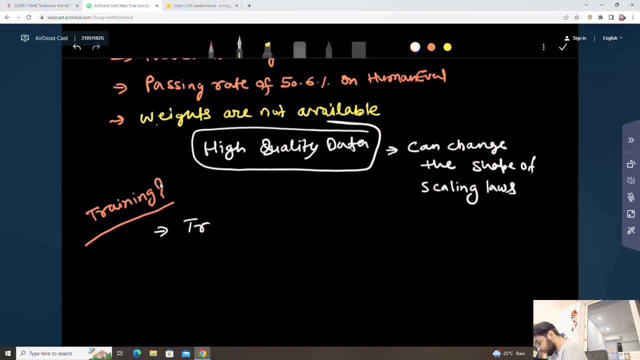 trained on a new data set with less than 7 billion tokens and it's really commendable to you know talk about it because when we when we talk about other lms that the number of token that they have used for at least in the training step it was more than at least 10 billion we'll talk about a lot of other models but trained on a new data set and they have used less than 7 billion token 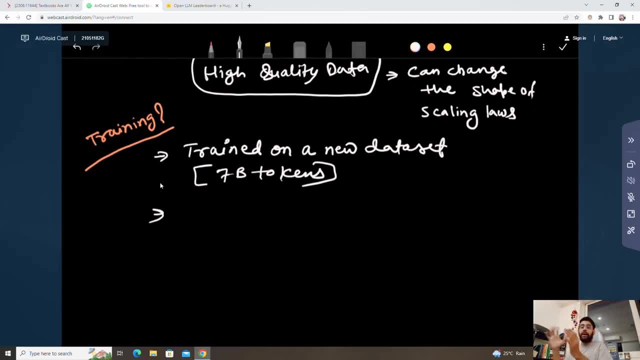 now they have basically divided into two steps I'll cover that the first step is to 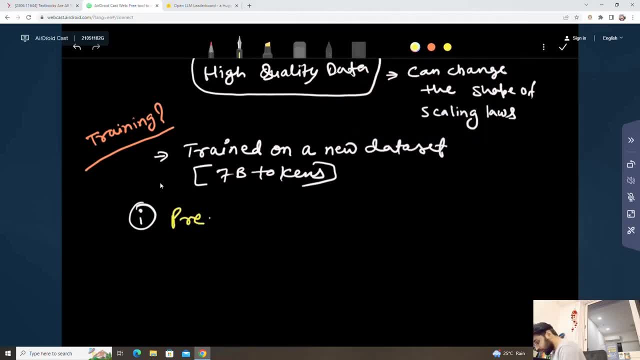 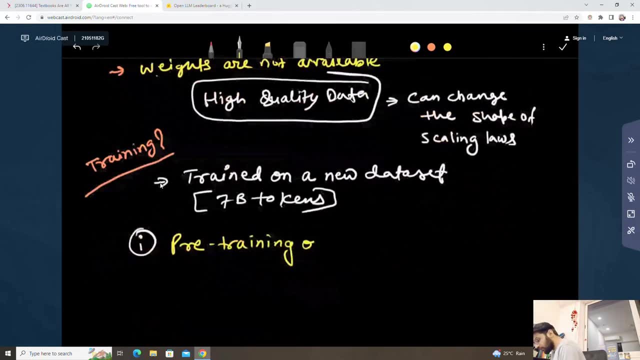 first step is pre-training pre-training on code textbook now this code textbook that we talk about right it's not a kind of an unified data okay it is combination of multiple data sources and also they have generated some data and we'll I'll I'll I'll cover that so what basically they have done in this case here guys on you know code textbook this basically is a combination of stack stack overflow 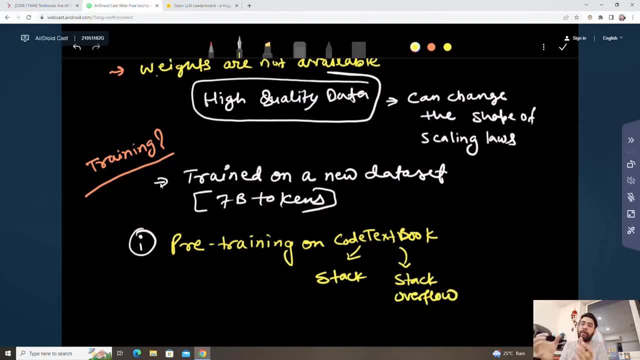 stack stack overflow and now they have generated some synthetic samples again using GPT 3.5 so you know and a lot of you know this kind of research that is happening 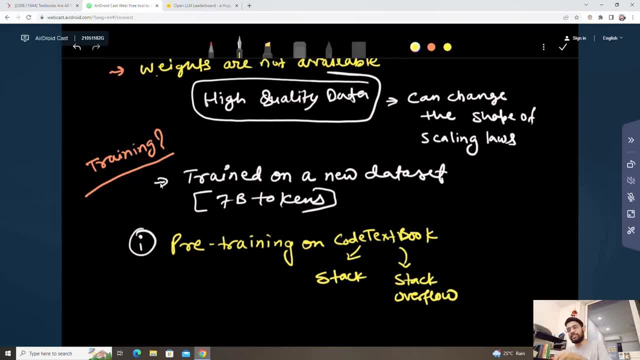 by GPD3.5 has been used to you know create or generate basically this data samples and it helps you generate samples very easily okay and it saves a lot of time so basically what they have done here they have also created synthetic samples synthetic samples generation 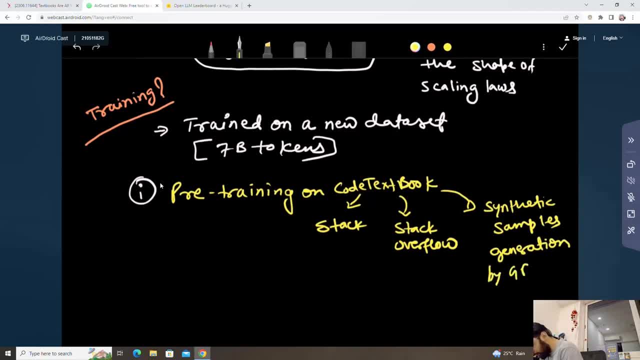 by GPT3.5 3.5 turbo so by GPT 3.5 so this was the step and the first step was on we talk about the data here 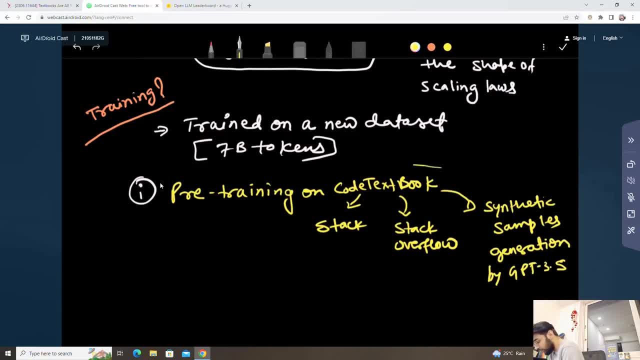 the pre-training on code textbook so this code textbook that you see it's combination of stack stack overflow the codes you know from the stack overflow and then the synthetic sample 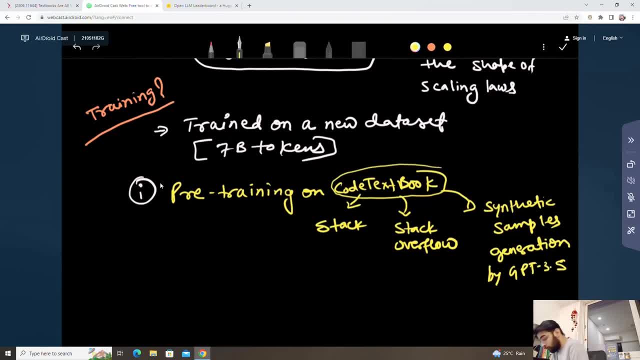 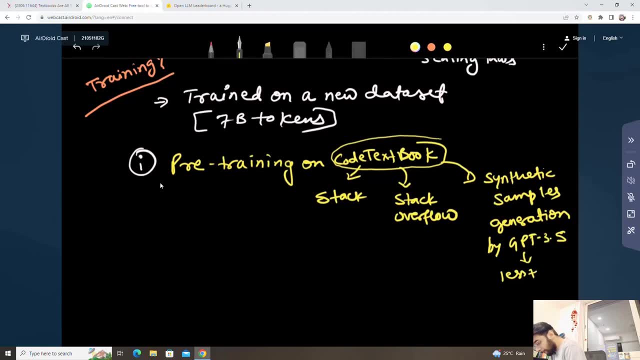 generation by GPT 3.5 and I forgot the exact number but I think it was less than you know 1B less than 1B tokens so less than 1B tokens okay this pre-training so this is the first step 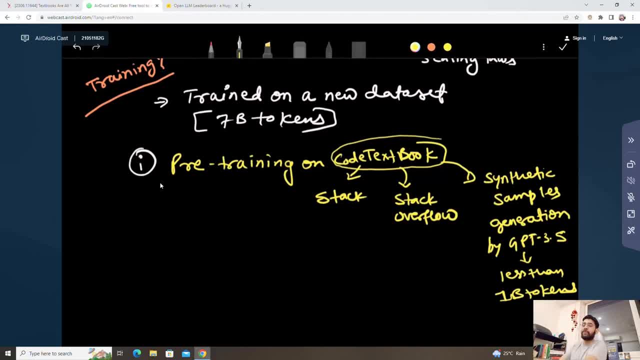 pre-training on code textbook that's what they have done okay and it has been entirely trained on a new data set they haven't taken any data set from hugging face data or any other data 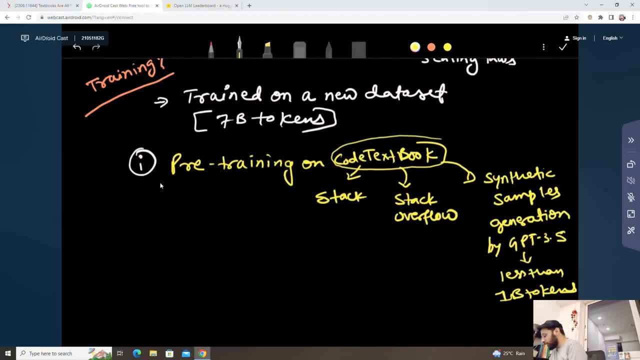 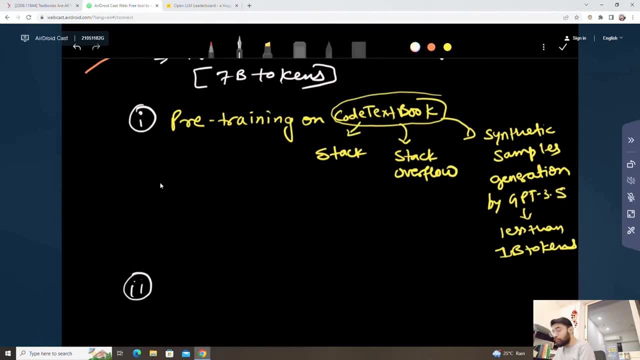 set in the community that is available okay they have trained on a new data set okay now the next thing is fine-tuning on code exercise 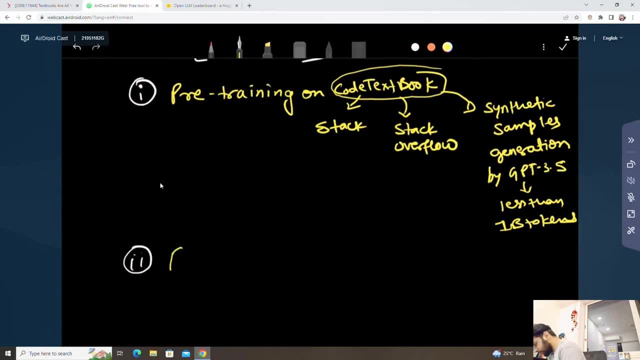 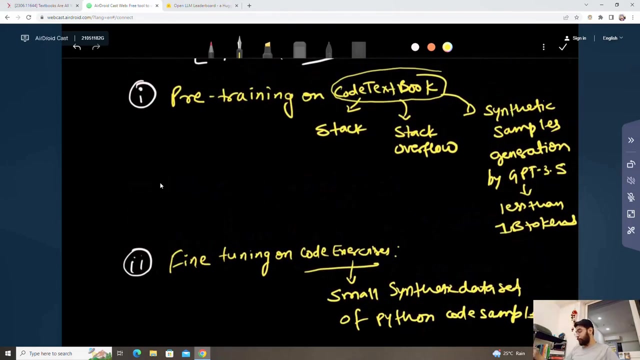 So what they have done in that case, fine tuning on code exercises. So in this they have a very small synthetic data of Python code bases, small synthetic data set of Python code samples. So this is a two step on the data part. So pre-training on code textbook and then fine tuning on code exercises. Now I hope you got at least the idea on the data part, what kind of data has been used to train 5.1 by Microsoft. 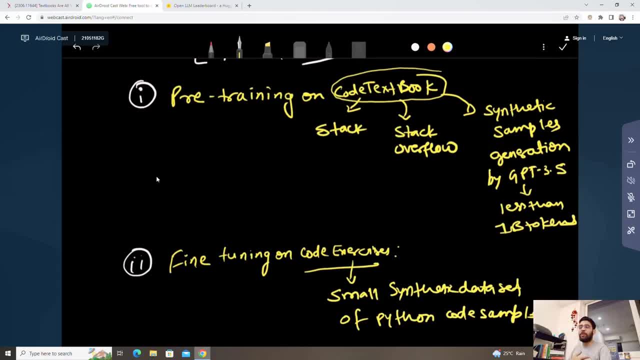 Which is very very useful. You know intuitive, at least for people like me who love AI, right. And if you come over here on this research paper, let me open the PDF by the way here. 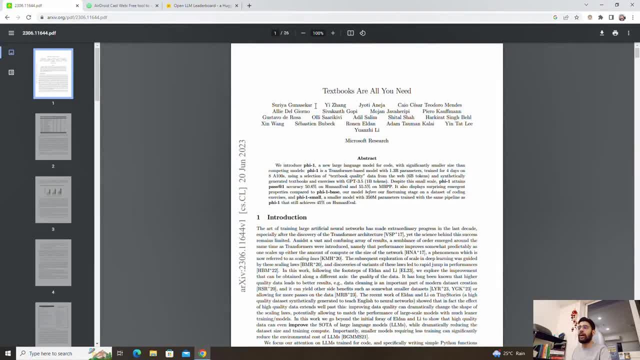 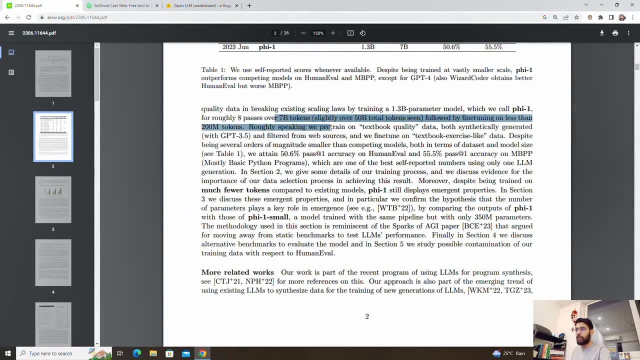 So I will just click on PDF and it will take me to textbooks are all you need. And let me just make it little bigger here. You can see 7B tokens, passes slightly over 50B tokens seen, called 5.1, passes over 7B and followed by fine tuning on less than 200M tokens. So you can read it over here. Pre-train on textbook quality data, both synthetically generated with GPT 3.5. 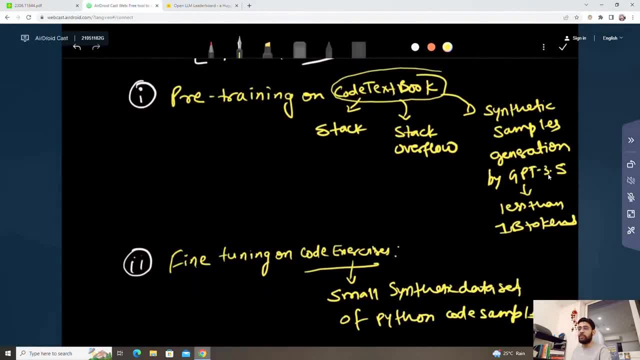 So you can see as I just covered right here on this cast by GPT 3.5 data. You can read that here as well. 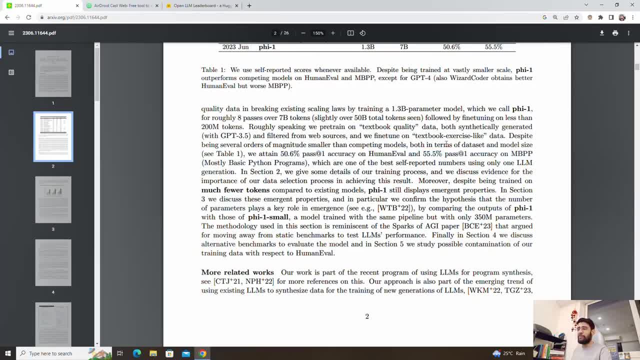 And then 50.6% on human eval, you know and MBPP, etc, right. So those things are still going on here. 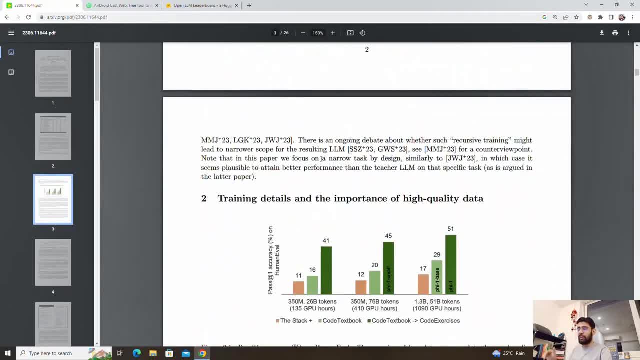 You can read that on a very high level and I will explain, now I will go to the training part guys, okay, after this. 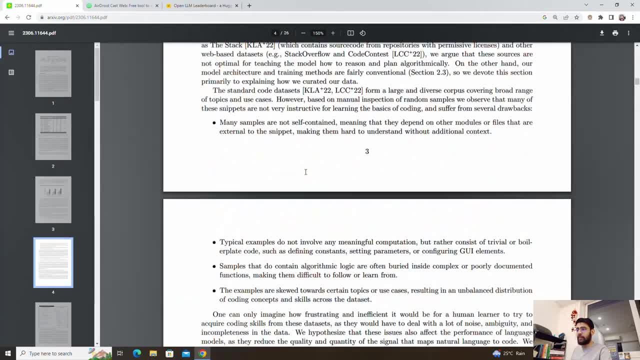 But before that we will focus on embedding. Okay. Now if you come down, you can just see the transformer based classifiers, etc, and everything. 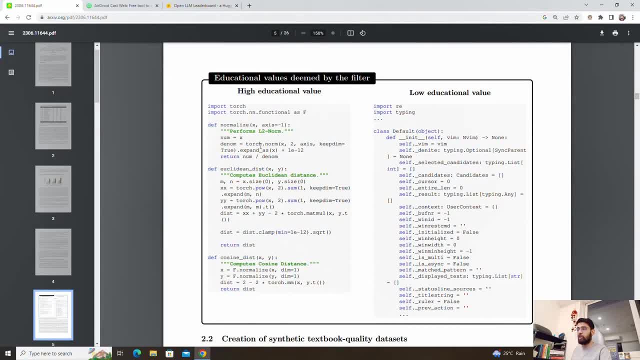 And this is the high educational value data over here, okay, define, normalize. And I will explain about this, that how, you know, techniques like rotary position embeddings, 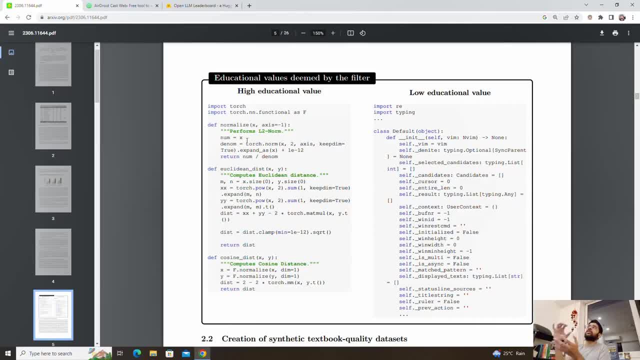 because it looks at the positions, because when we talk about normalize, it looks at the position of normalize, okay, in the training step. So we will cover that as well. 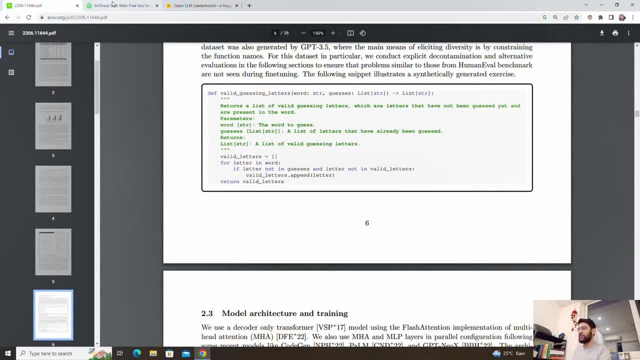 So very, very interesting. Very, very interesting research effort guys to read. So let us move on now, okay. So this was in the data part, so preparation of data. 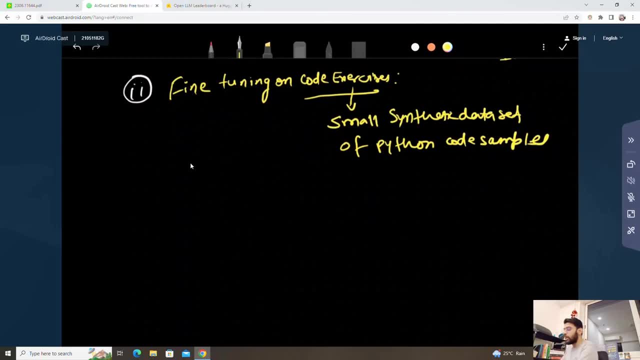 Now once they have this data ready, the next step that comes in on that is embeddings. The hot cake right now, when we talk about building large language model based solutions, we call it embeddings, right. 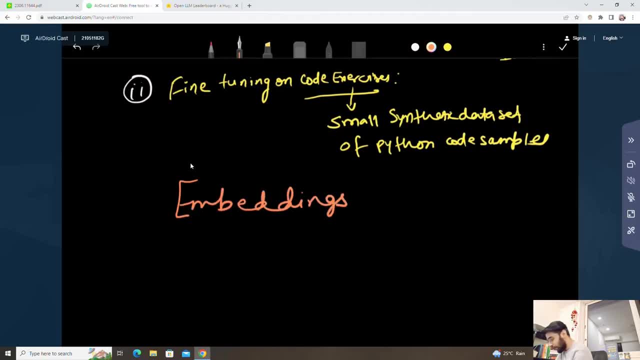 So let me write it little in big font size, embeddings. So now once they have the data, okay. They have the data with them. 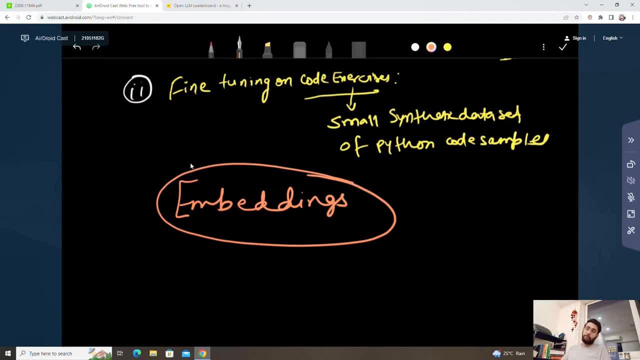 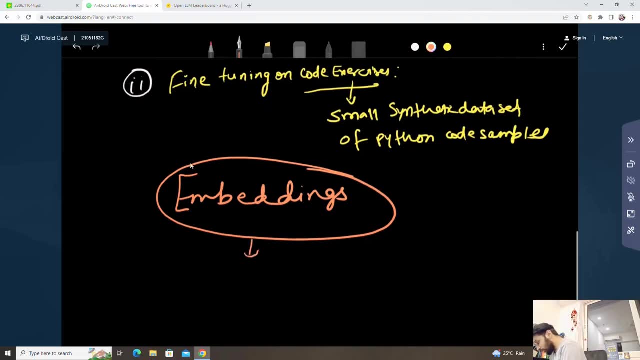 Now they have to create these embeddings, okay, on top of that, right. And that's where they used code gen, okay. And that's code gen has been used here, okay. 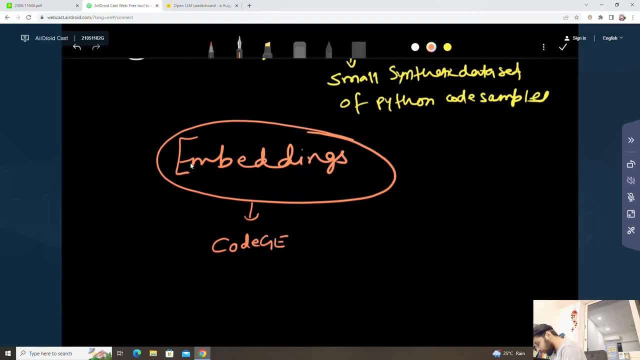 So let me just write code, code gen has been used basically to create the embeddings. So let me just write it over here. Create the embeddings. Okay. So, okay. Okay. Okay. Okay. Okay. 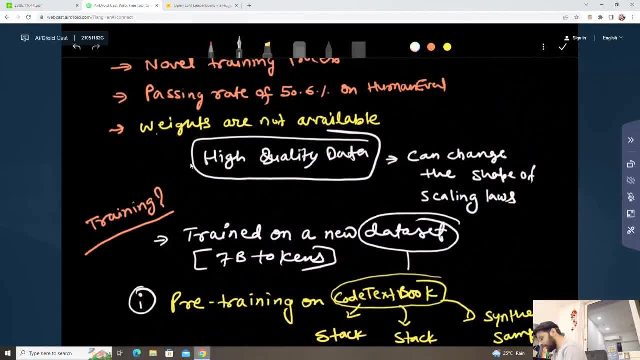 So now here is the data strategy. So this was basically the data sets. So let me just write data sets and our data sets, we have the embeddings part of it. 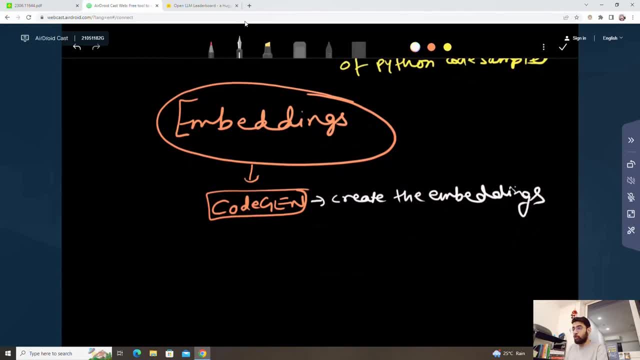 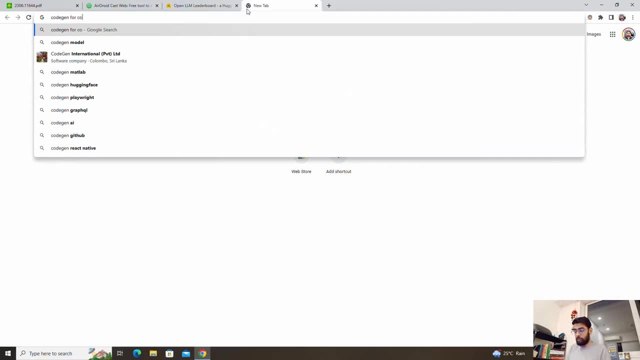 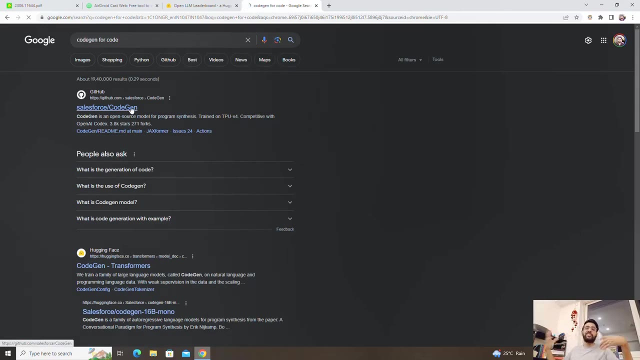 Now create the embeddings using code gen. If you are not familiar with code gen, code gen has been used basically, you know, let me just write it for code. It has been the most used, okay, model right now for synthesizing the programs by Salesforce. 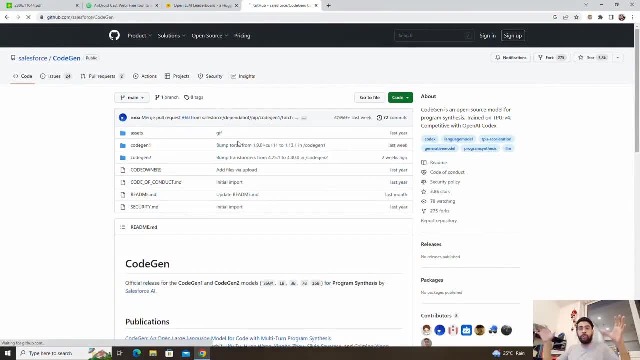 And Salesforce, I think deserves, okay. It deserves a lot of credit. 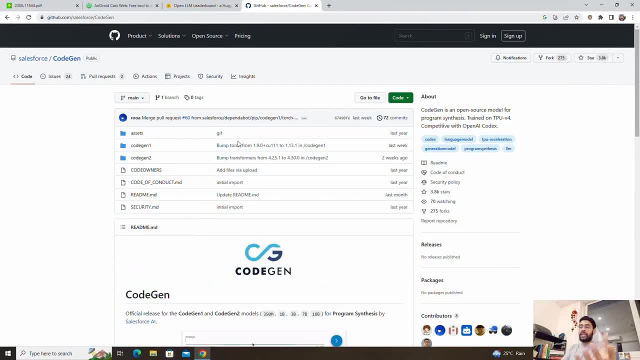 I don't know. People, I don't see researchers talking about Salesforce because they have done a lot of things for open source community. 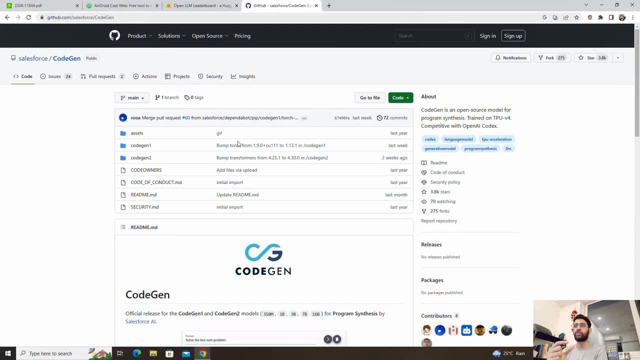 Okay. They, I think the model blip is also from Salesforce. Let me just check it out. Okay. The, the blip model. 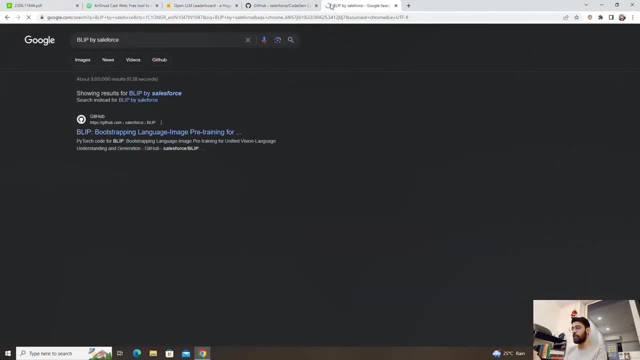 So I'm just writing blip by Salesforce and it will show me if I'm wrong there. Okay. So if it, it might say, yes, it's by Salesforce itself. 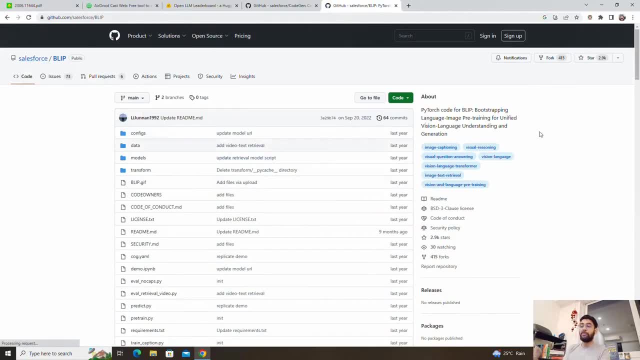 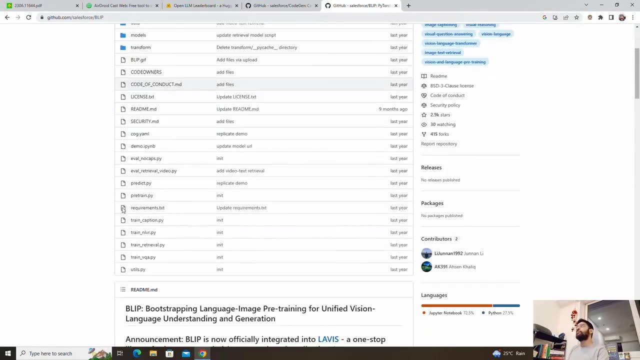 Okay. You can see Salesforce blip. Bootstrapping language. Image pre-training for unified. Vision language. So blip is very, very fundamental when you talk about, you know, uh, uh, VIT based models, right? Vision image transformer. Okay. Blip plays a huge role over there. Okay. And that's again by Salesforce. 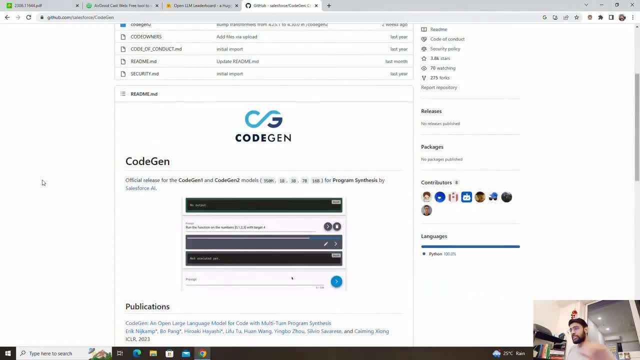 Salesforce has code gen and Salesforce has other open source model and they deserve a lot of credit that empowers the open source community and research like five one, for example. So, you know, code one has been used to create the embeddings. So you can also have a look at code one. I will give the link in the description guys 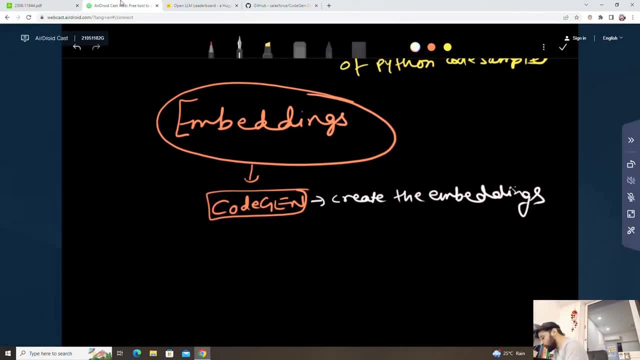 Okay. So code gen. 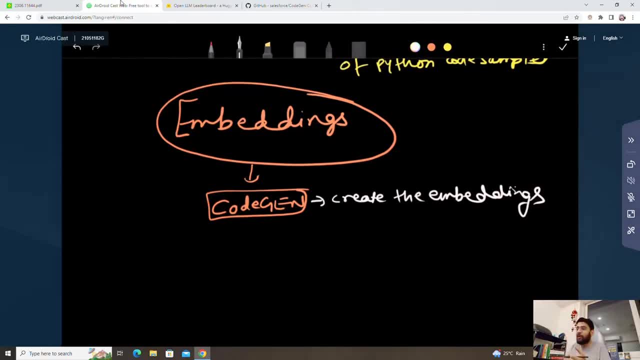 Now, once we have the embeddings, how will you find out that, right? These, uh, embeddings kind of, you know, like we have to predict the quality of each samples. 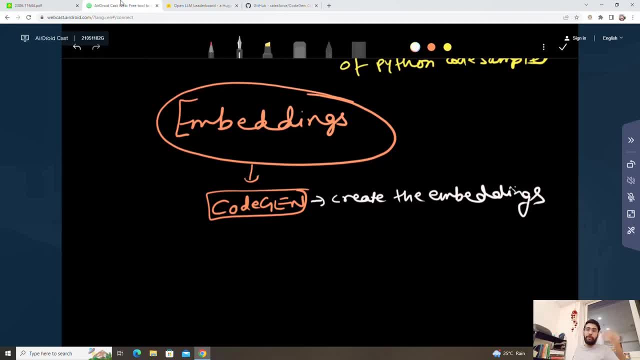 Okay. If the qualities are even good or better or something. Right. So you need a classifier now. 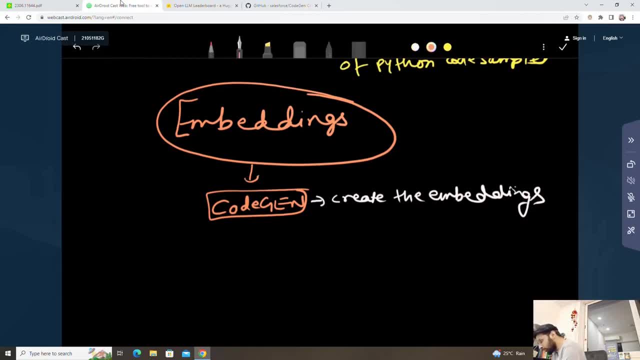 Okay. So they have used, let me just write it over here. They have used again, uh, random forest. So random forest classifier. Okay. So random forest classifier has been used. 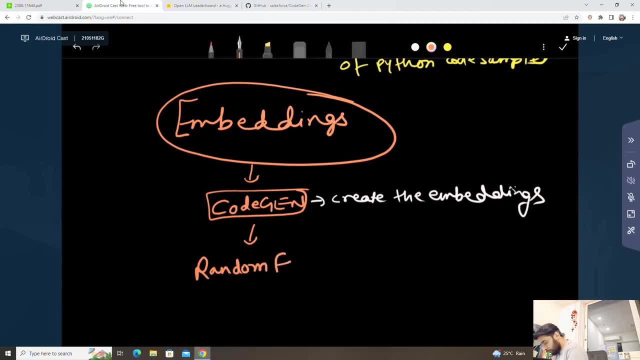 So now we have a data, the embeddings with the code gen and now with the random forest classifier. Now what it does. 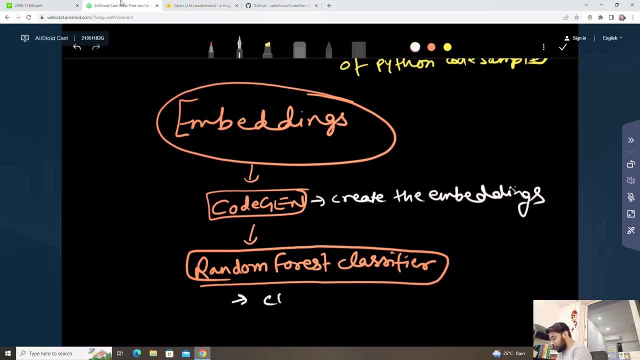 Okay. Let me just write it over here and basically classify classifies, okay. Classifies to basically classifies for quality of code. Okay. So now we have a data and embeddings. 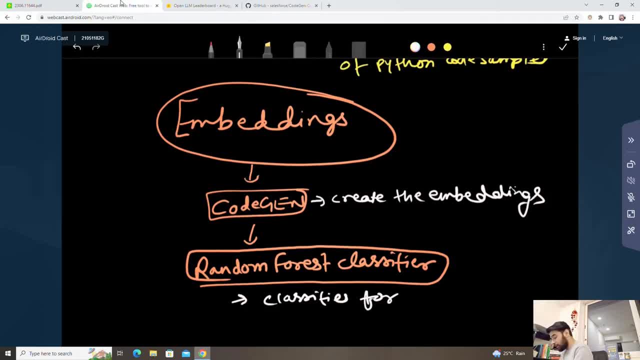 for quality of each sample for quality of each sample so quality of each sample now this is what it does okay so now till now we have discussed about the process so we have now the other let 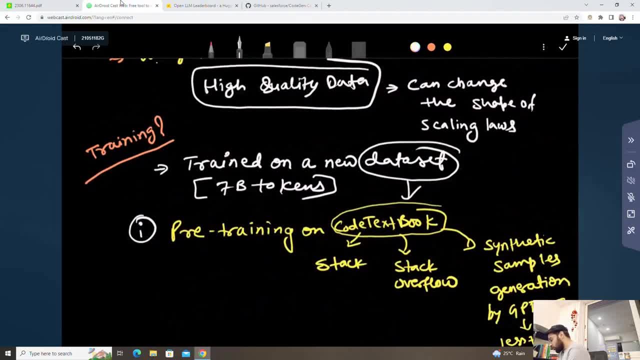 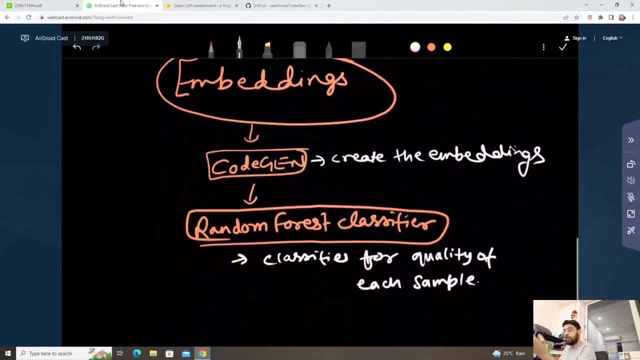 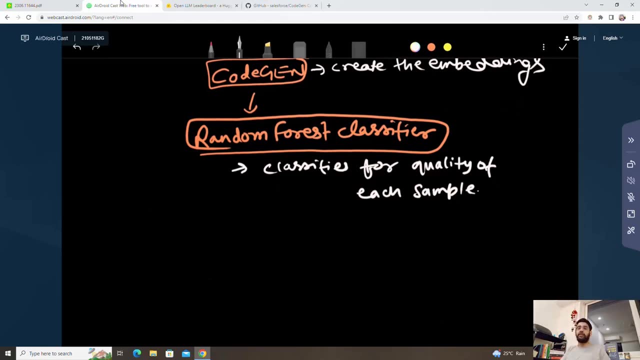 me call it training 5 1 5 1 turning so we start with the data set and then we move to embeddings using code gen now we we have this now what we will now discuss is in detail that how the training has been done which is the novel approach okay of training these guys okay so let me just 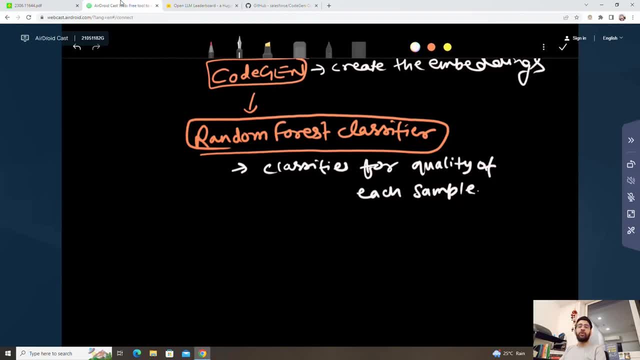 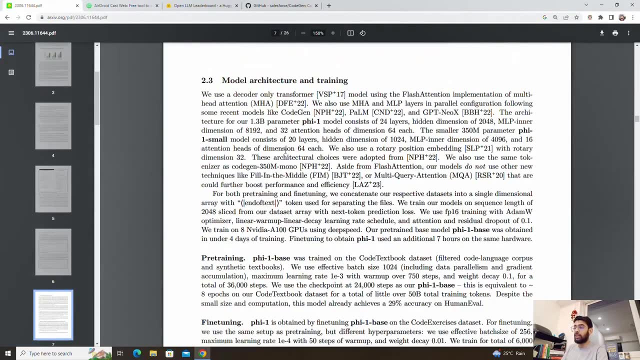 give you you know a high level view of that and you can read the research paper and you can come up with your findings i have read it and you can see the model architecture and training so we'll 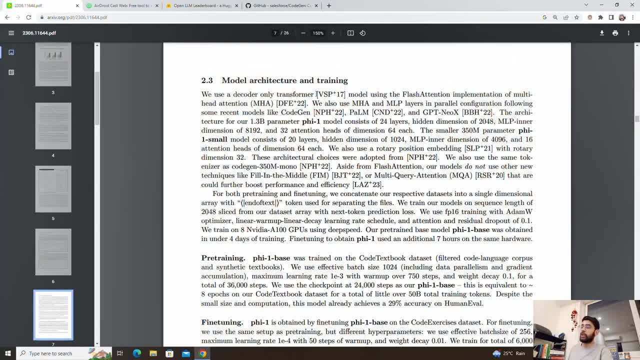 now deep dive into it we'll understand what they are talking about mha which is multi-head flash attention implementation of multi-head what does it do basically and what does the rotary and position embeddings and this mlp layers what are they doing inside this okay so we'll 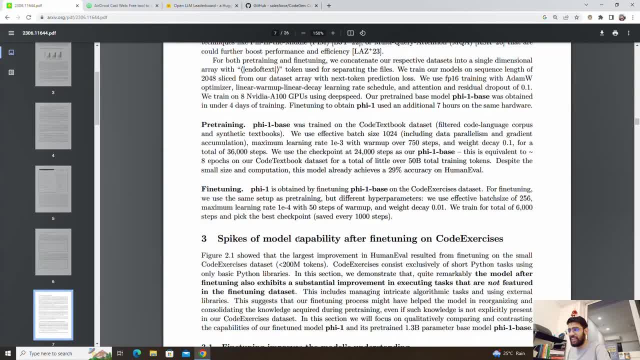 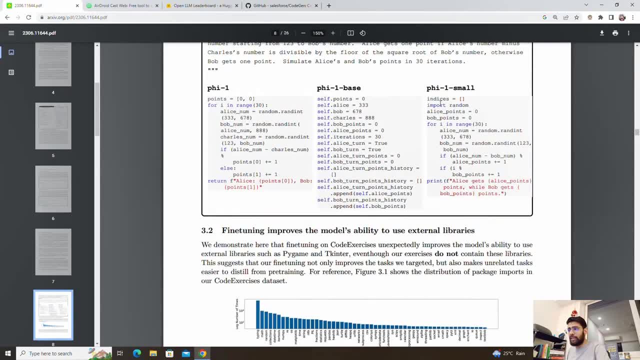 discuss about these things you can read it over here the pre-training and the fine-tuning etc etc so let's understand so you can see 5 1 5 base and 5 1 small three different types of weights 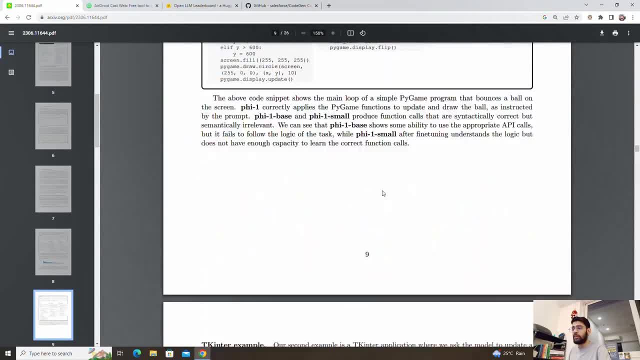 okay that they have they will i don't know if they will make it available for public use but they will make it available for public use so let's understand so you can see that they have they will make it available for public but that's okay that's not our concern 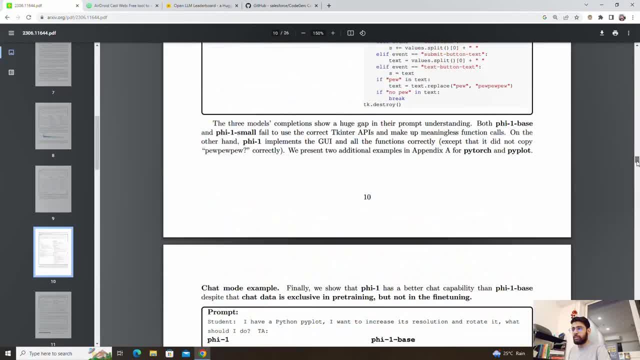 at this moment and so i'm not going into the evaluation part now let's see okay so i'll break 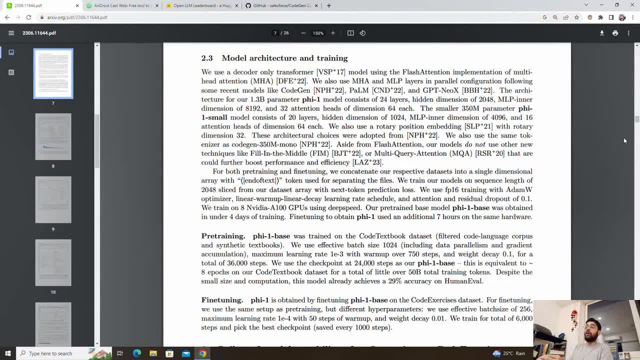 it down okay the model architecture and training it's a decoder only transformer model so let me 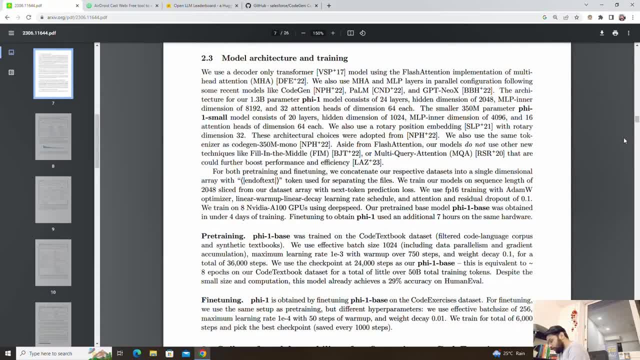 write this guys okay so let me write it for you so it says decoder only transformer model using 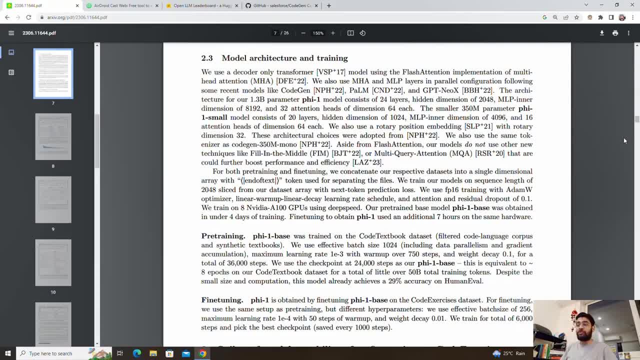 the flash attention very big you know this might sound very big but it's actually being used actually 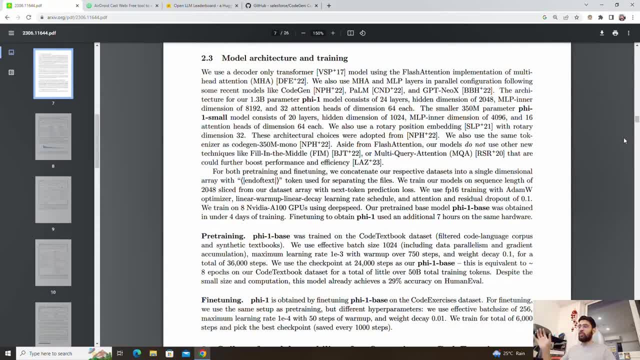 big words to you okay but it's a very intuitive okay so decoder only transformer vsp plus 17 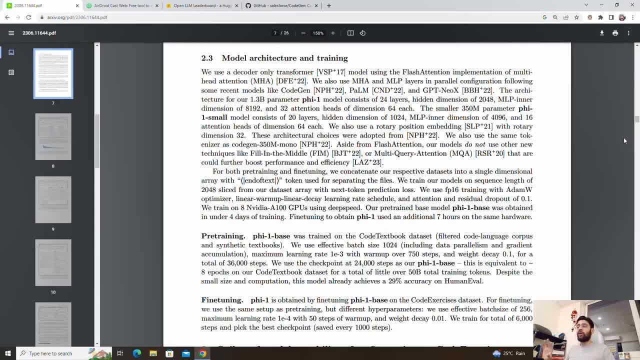 model using the flash attention okay of multi-head attention we also use mha mlp layers in parallel 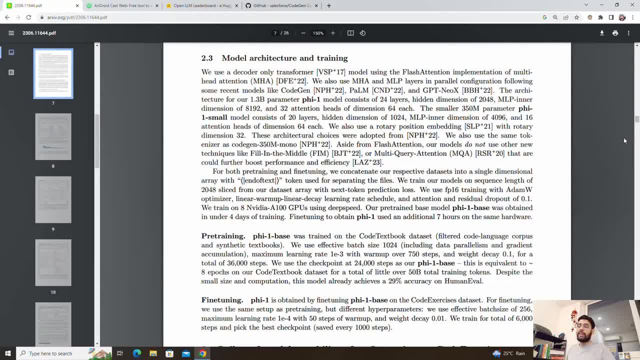 configuration okay following some recent models like code j and palm and gpt new okay 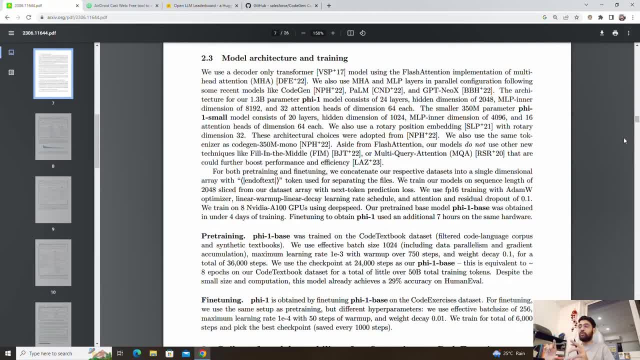 we also use a rotary position embeddings with rotary dimension 32 let's let's break it down 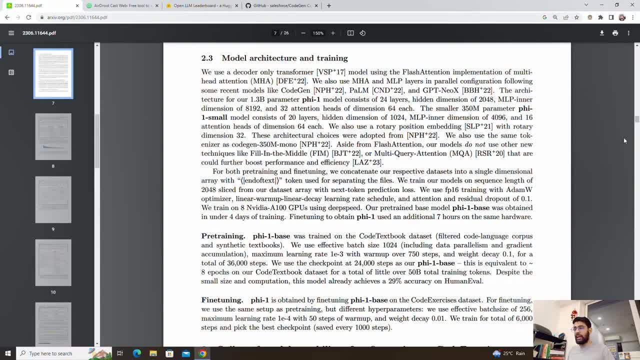 okay so i have done my study on it and i will break it down and help you understand 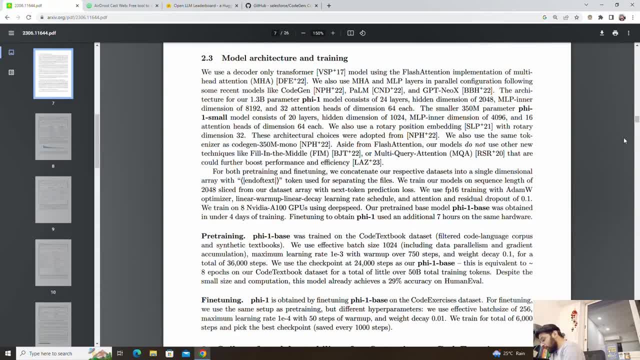 okay and how so let me first write it down so we'll start with tokenizer 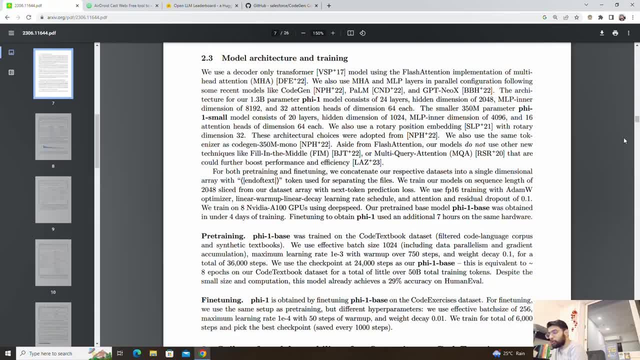 maybe in the very lemon term okay the state goes like this we have a tokenizer and then we and we'll go into detail okay rotary position embedding let me first write all these terminologies okay rotary position embeddings and then we have flash attention then we have flash attention then we have you know multi-head attention so multi-head attention and then we have uh parallel mha and mlp so let me just write it as well here parallel mha and mlp layers so i'm just going to write it down and decoder only transformers i'll just write a different color because that's how they define this model decoder only transformer so that's the step okay so this is what we have so we have tokenizer rotary position embeddings flash attention multi-head attention parallel mha and mlp layers decoder only transformers how can we explain these guys now okay But before that, I'll also explain, I think you should know a little bit about the hyperparameters. And then we'll deep dive into, you know, about this detail. So let me just, let me first explain in that. 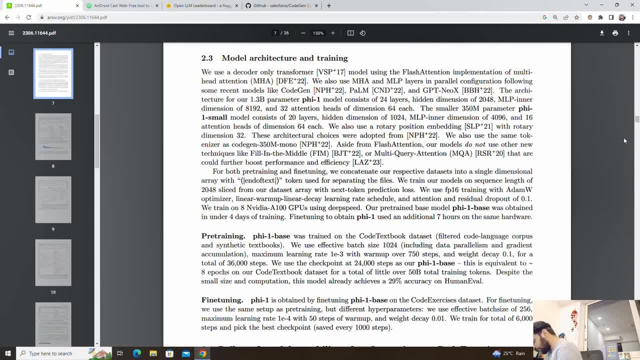 Okay, so the first is layers. The first thing is layers. How many layers? Okay, when we talk about 5-1, okay, or 5-1 small. So we'll talk about these two models. The one is, let me just write over here. So let me just, so I'll just write 1.3 billion and 350 M. Okay, and then we will Okay, and then we will Okay, and then we will 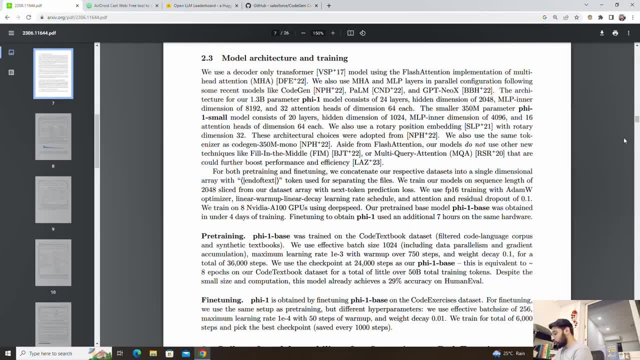 put our hyperparameter over here. Okay, so let's write now. So the first thing is layers. So on the layers part, okay, for 24 layers, for 1.3, 1.3, which is 5-1, and then 20 layers for 350 M, M weights for our model. Okay, so 24 layers. 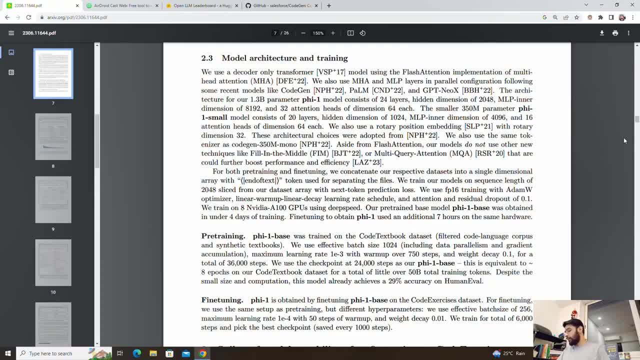 Okay, so 24 layers, 1.3, B, and then 20 layers, 3.8. So basically, it's, it basically refers to the number of stacked transformers layers. So we have transformers layers. So the number of stacked transformers layers in the model. Okay, that's what it represents, basically. Maybe I can write it down quickly. So, you know, refers to, refers to the number of, you know, stacked transformer. 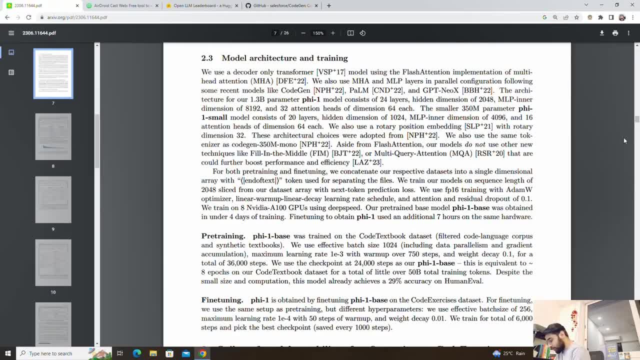 Stacked transformer layers in the model. So layers in the model. So the first part is layers. Okay, so we have, we are currently looking at the hyperparameters, and then we'll deep dive into the step to understand that which one has been used where. Okay, and then we have something called hidden dimension. 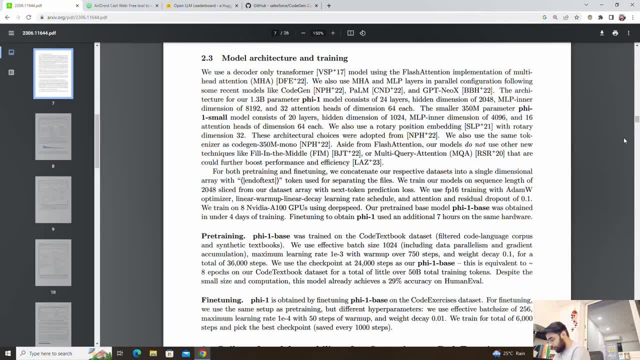 Now, for 1.3 B, and 350 M. 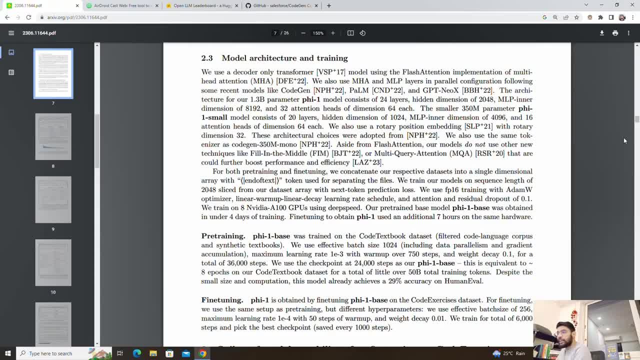 So for 1.3 B, the hidden dimension is around 2048. You can see it over here. If you see this, it says hidden dimension of 2048. So let me just write it 2048, and for 350, it's 1024. Okay, now what does hidden dimension do, guys? It determines the size of the vector representation. 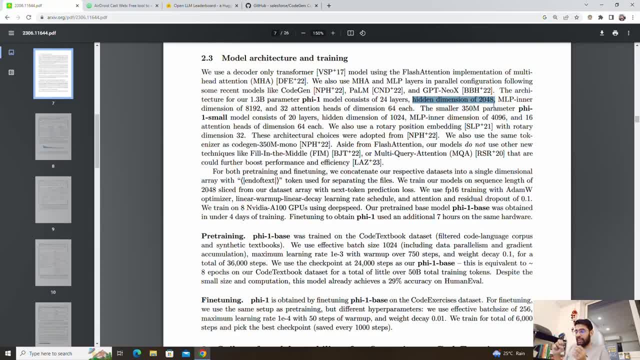 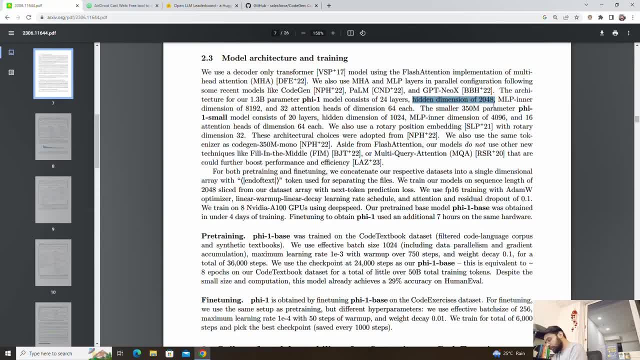 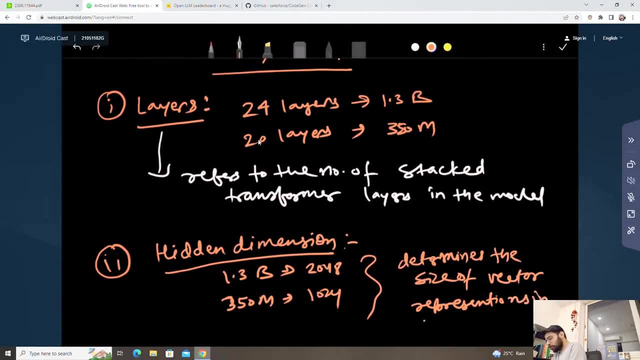 So vector representations. Okay, let me just go back on the cast. Representations in the model. That's on the hidden dimension now. Now, what else we have? We have MLB. 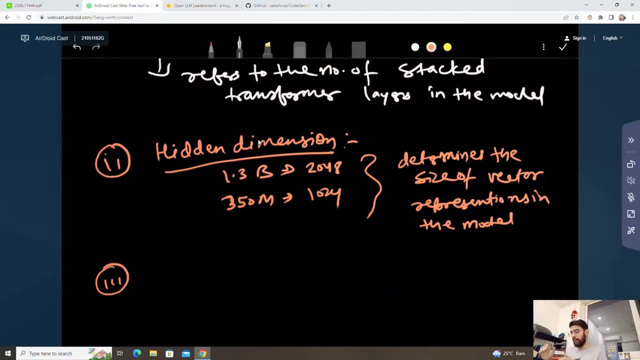 We have MLB inner dimensions, the multi-layer perceptron. Okay, and that's inner dimensions. So MLB inner dimensions. 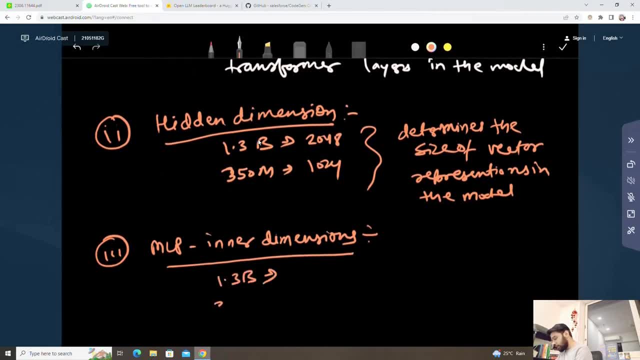 So for 1.3 B, and 350 M. So for 1.3 B, it's 8192, and for 350 M, it's 4096. 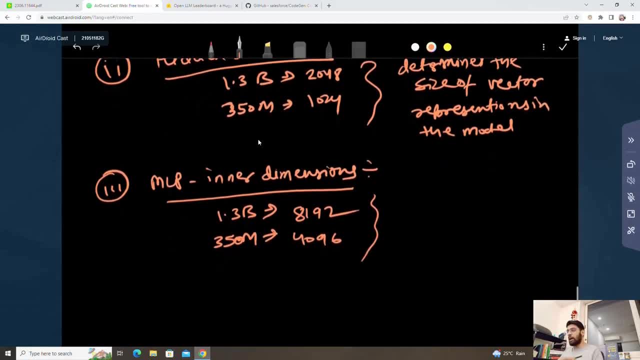 Now, what does MLB inner dimensions mean? What does MLB inner dimensions mean, guys? It's basically size of, you know, intermediate layer within the multi-layer perceptron. 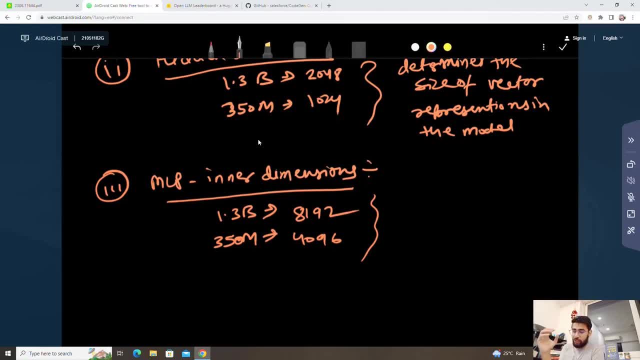 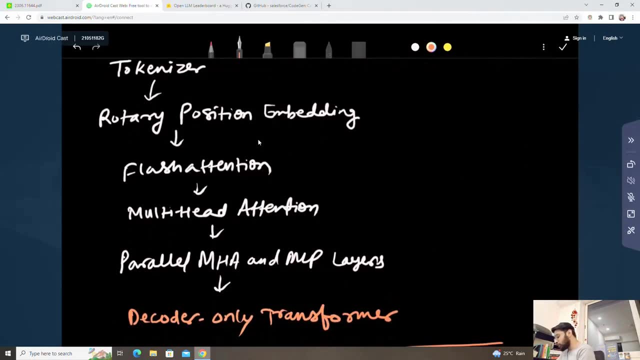 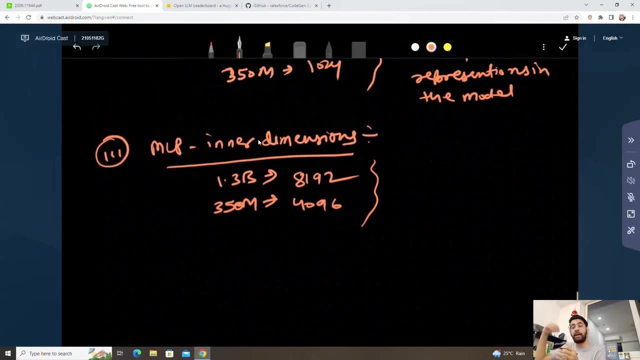 So we have MLB is there, right? MLB component of this model, the 5.1 model, because if you see here, if you go up, it says parallel MHA and MLB layers. So there are MLB components, there are MHA components, and for that MLB components, we have inner dimensions of this MLB layers. Okay, so these are basically size of intermediate layers. 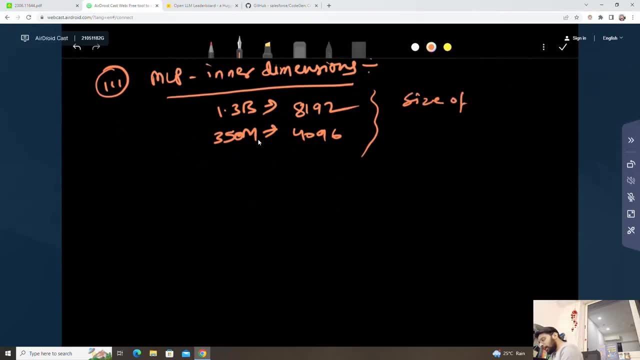 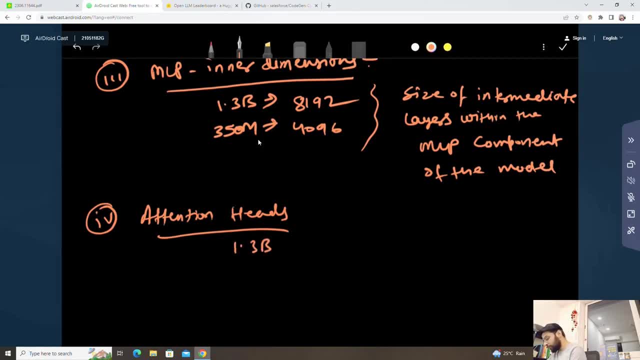 Now, in attention heads, for 1.3B, and let me also write 350M, for 1.3B is 32 attention heads, 32 attention heads. And now these attention heads will also have their dimension. Okay. So 32 attention heads, I'll just write H, with a dimension of, with a dimension of, with a dimension of 32. 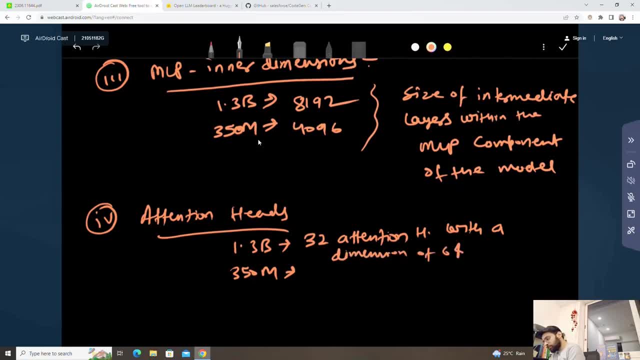 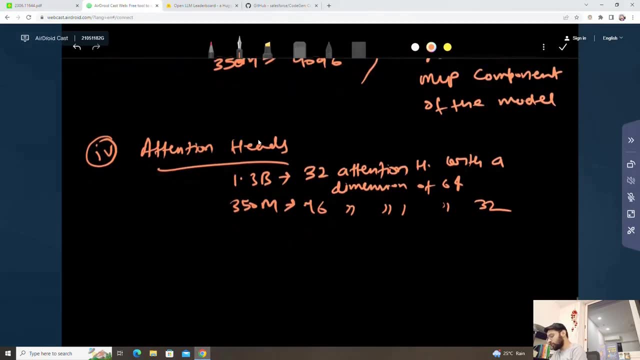 dimension of 64 and for this 350 it's 16 attention so let's write 16 attention head with a dimension of 32 just half of it okay so basically you can just see right on the on the weights that we are 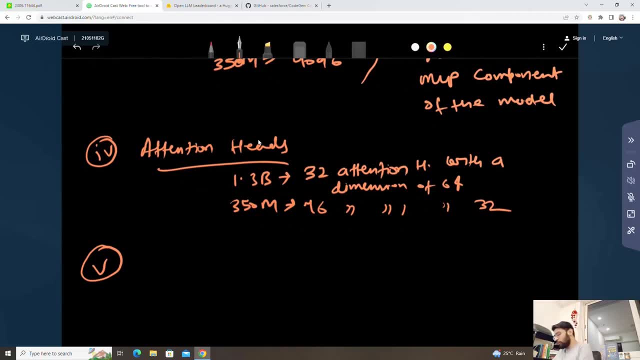 talking basically it's half of its values there now we have sequence length so what does what do you mean by sequence it basically it's fixed at 2048 it's come to fixed and nothing but the 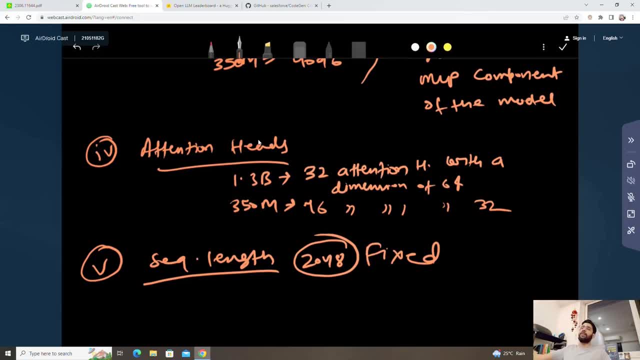 maximum number of tokens we are talking about you know when GPT 3.5 3 it was around 4096 alert or 2048 or something then it increased to 4096 and GPT 4 can also take around I don't know it's in more than 10,000 if I'm not wrong let me know okay how much token it can take so maximum number of 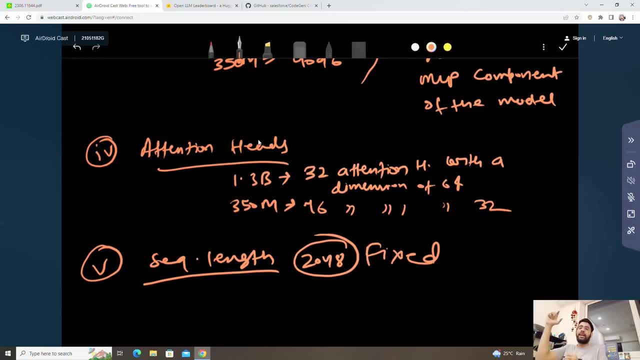 token the model can process in a given code snippet so you are writing the code snippet 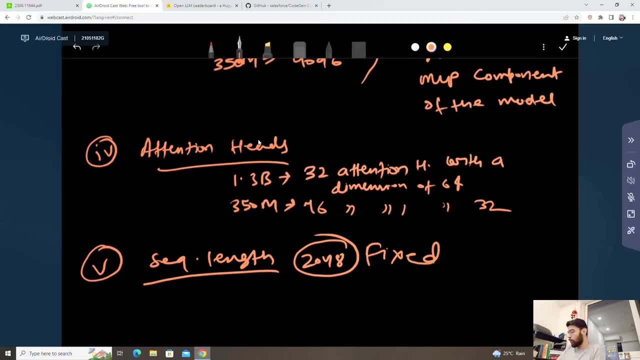 right it's the length of the code that is being processed in a given code snippet right it's the length of the code that is being processed in a given code snippet right it's the length of the code that we're talking the maximum number of tokens okay so unique tokens by the way okay so maximum number 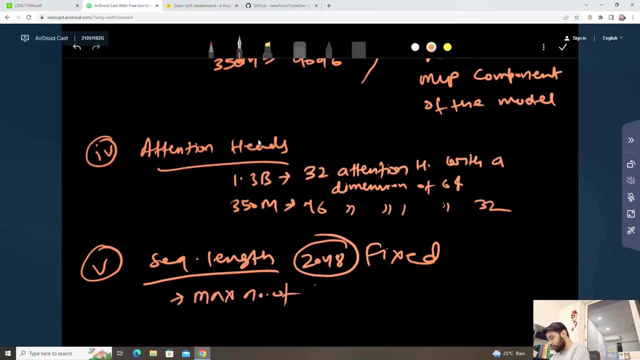 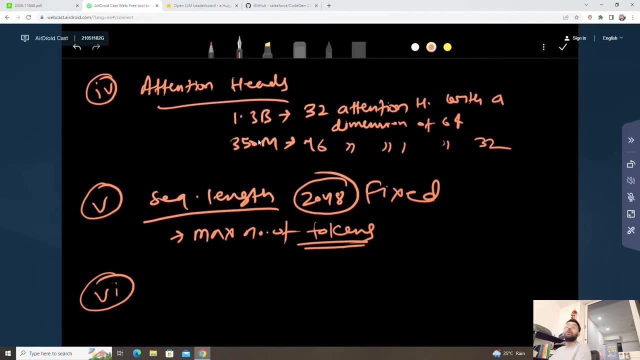 of tokens no it's not unique tokens unique tokens in the training process but when you are making 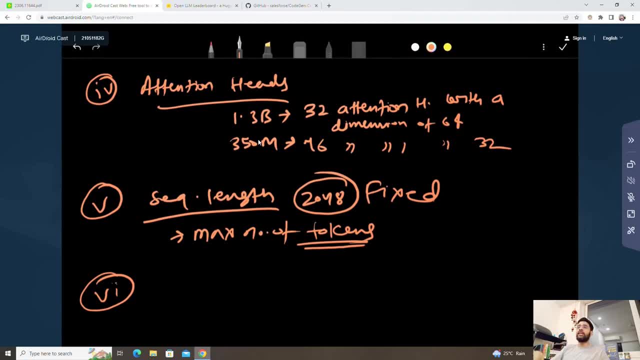 the request so model can generate some code or output for you then it doesn't look at the unique tokens so maximum number of tokens can be 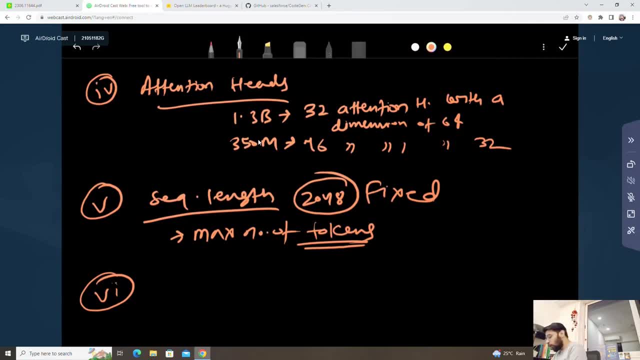 easily brought in in the training process okay so maximum number of tokens okay so maximum number of tokens can be generated and a minimum number of 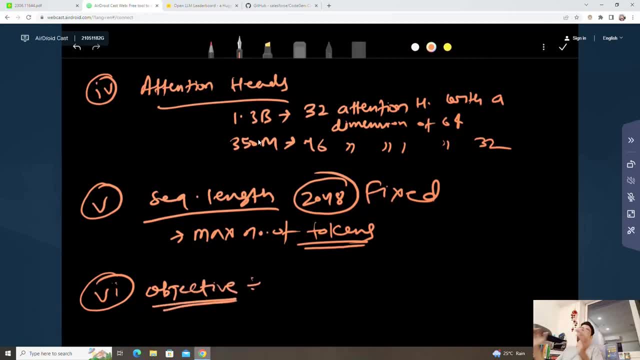 tokens or user knows okay but maximum number of tokens that can be generated 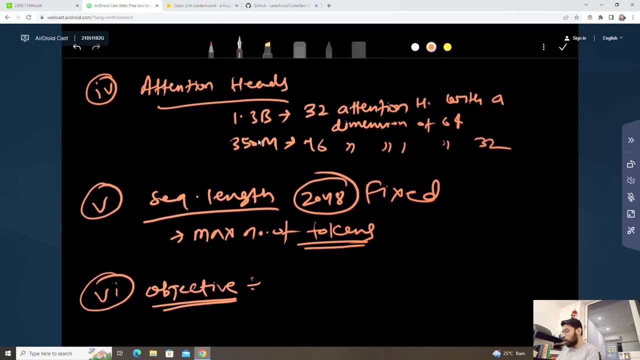 using the flow cost method that is being brainstormed to generate the 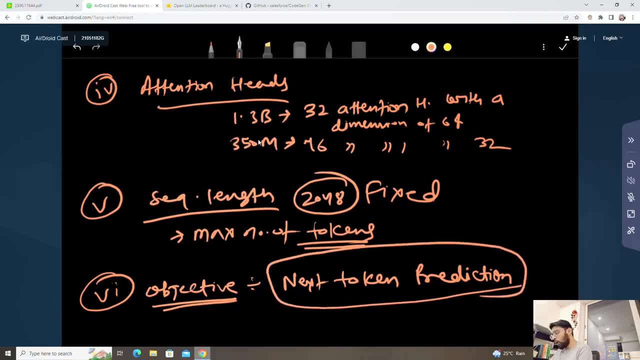 desired conclusion what you see on the left is the variable tables one by one you see that as we have now which is basically you know this is the way in which your model is creating the hardship in a given or also in the unreal mode so stories that you need to further understand this kind of patterns you need to so 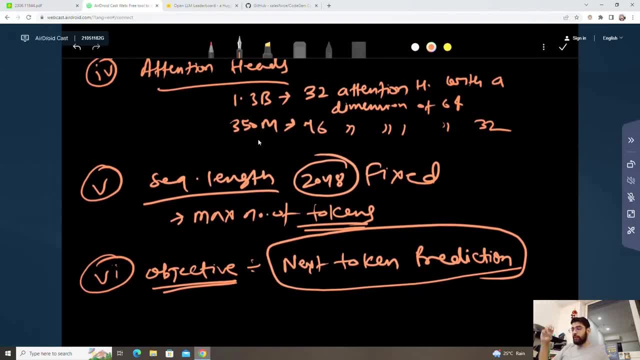 next token in the you know code sequence given the preceding tokens so these are the hyper 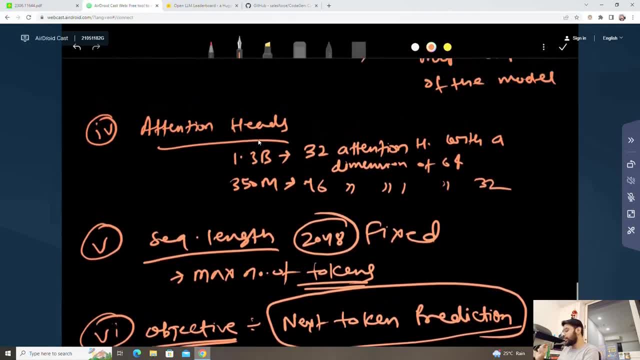 parameter for this model so sequence length objective attention heads mlp inner dimensions 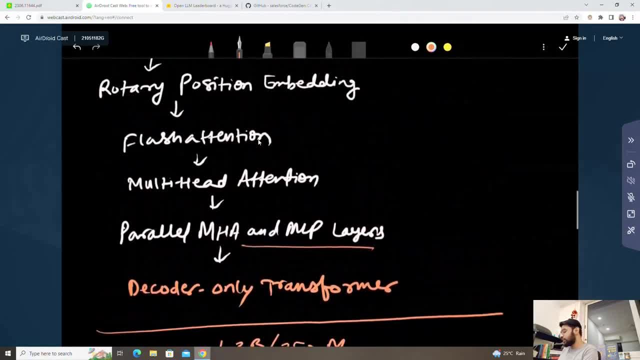 hidden dimensions and layers okay and these are these are the steps in the training process tokenizer i don't know if i should explain you because it might be very lengthy if i explain 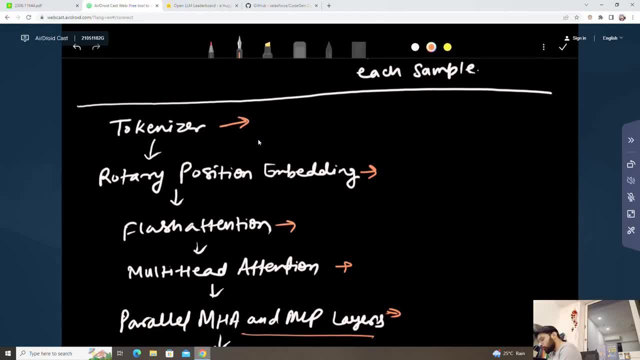 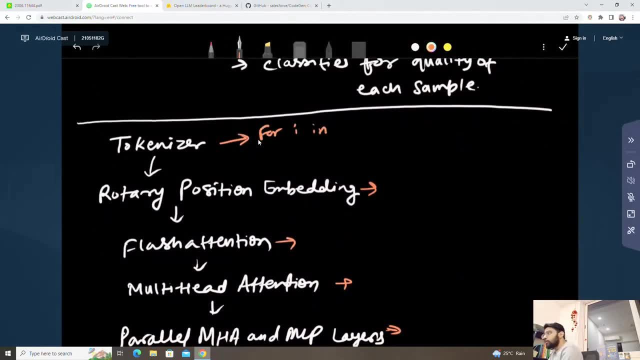 okay let me watch very quickly okay so what do we what do we make tokenizers for example let me just do here so when i write for i in range so i'll write write something for you guys so for i in range and i write something like this if this is my basically the code snippet okay example okay so how does tokenizer basically breaks it so basically it breaks it into tokens and for this case the token will be you know like for and next token will be i the next token will be in the next token 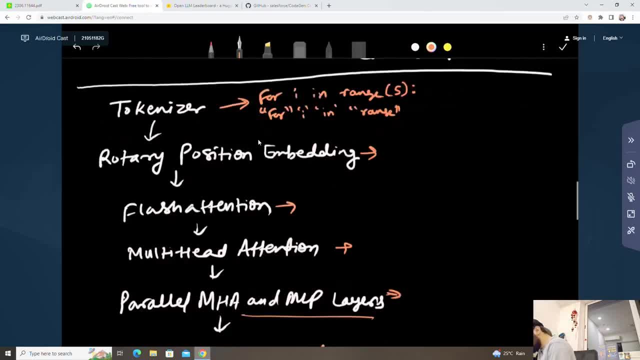 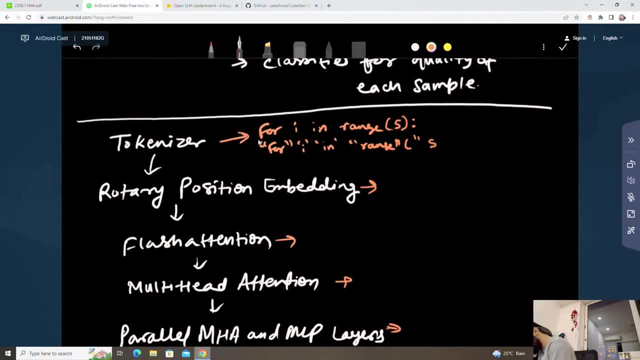 be in range something like this right and the next token will be this excuse me and this next token will be this parenthesis and then five so every token that you see right basically breaks into the token that's the first step tokenization okay the tokenizer 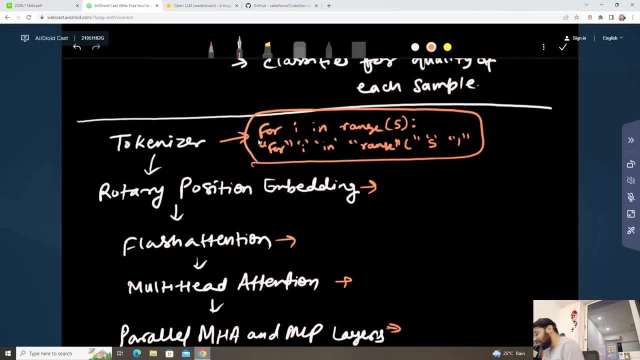 but rotary position embeddings is you know is very very intuitive to understand guys 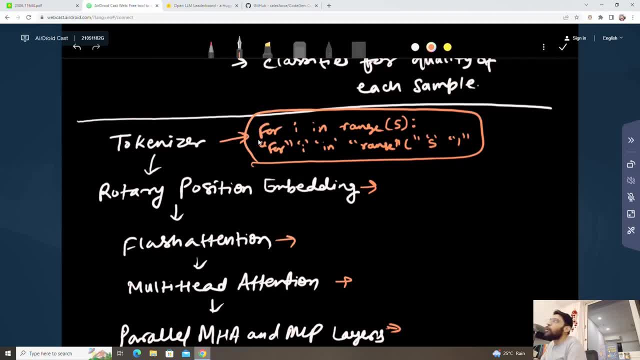 rotary position embedding so it's basically help the model understand rotary position embeddings you can see the position right it basically helps the model to understand the position of the variable that's what it does so for example if i write here 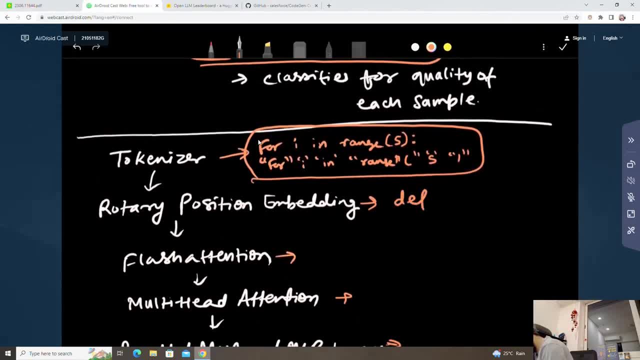 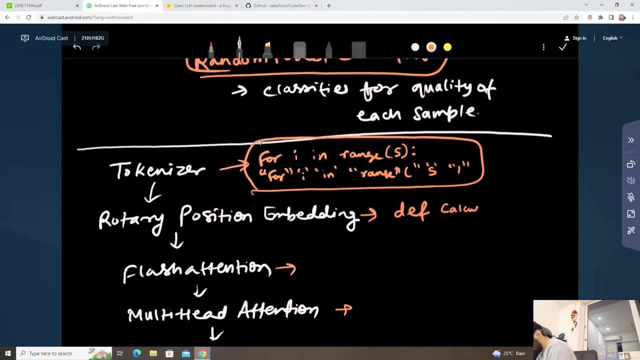 of a code snippet so let me just write so i'm writing define so basically defining a function in python so define basically calculate so let me just write define and calculate underscore number 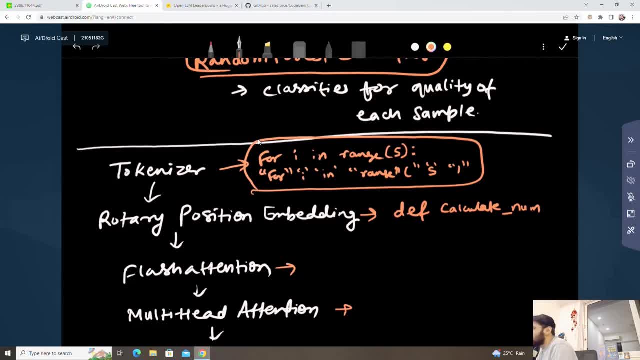 or num and i'll just put it over something like or let's keep it like this you know number i'll just put something x over here okay calculate number i'll just put something x over here okay 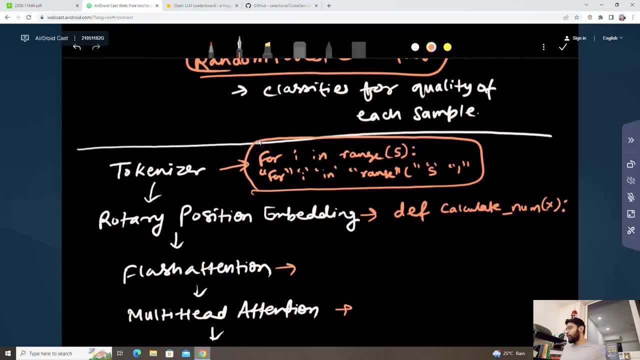 calculate number x or calculates whatever it is okay the code snippet now what it does guys okay 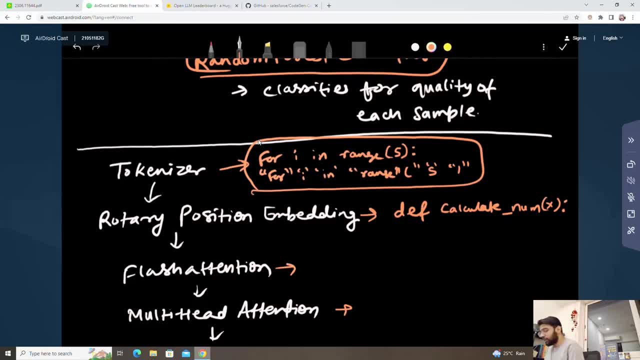 model to understand the variable num okay with the variable x by the way sorry the variable x 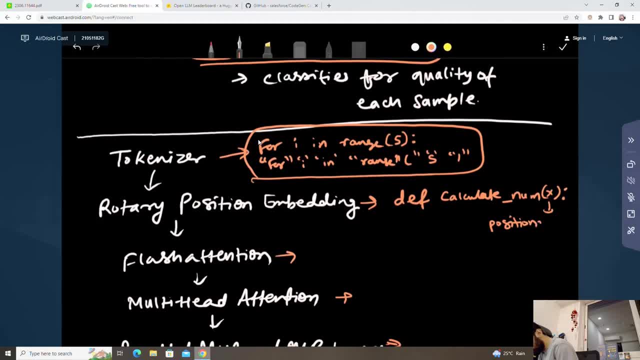 so positioning of positioning of variable x 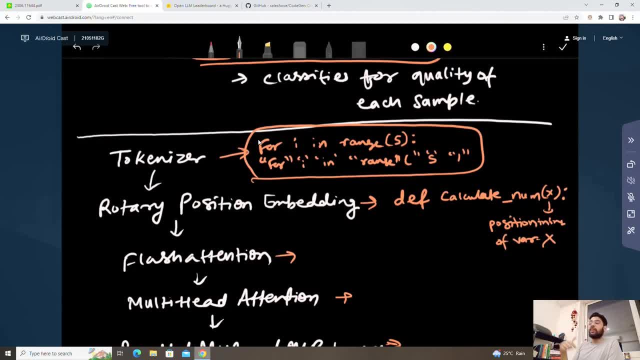 that's that's how we do rotary position embeddings but it's a very uh complex topic uh to be honest when you talk about a rotary position embedding because they use kind of some kind of trigonometric function there's a lot of things goes up you know 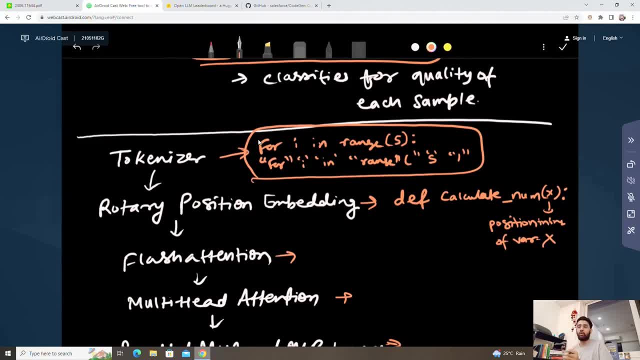 behind hood of rotary position embeddings let me know if you want me to have a video on this steps subsequently right or i don't know if i can cover it in one video right it might be long so for this step uh rotary position embeddings of flash attention i can have a 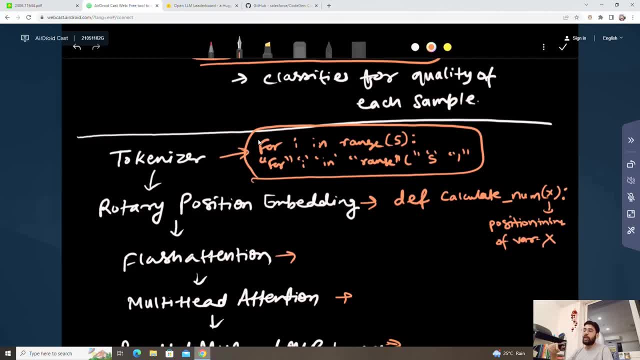 separate video let me know your views guys if you are interested if you if i get some good you know feedback or some appreciation on this video i might create a video for you guys on 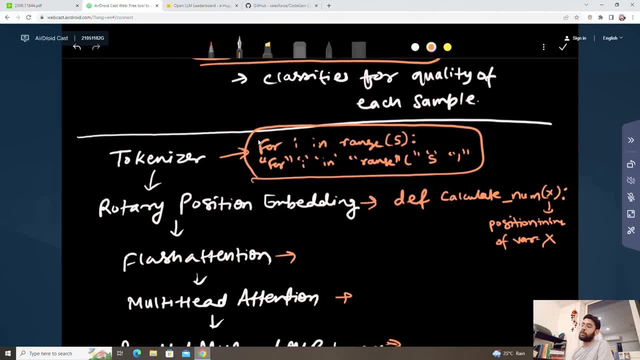 explaining in detail with some examples and in very layman terms like what we mean by rotary position embeddings and flash attention for example so let's let's understand the flash 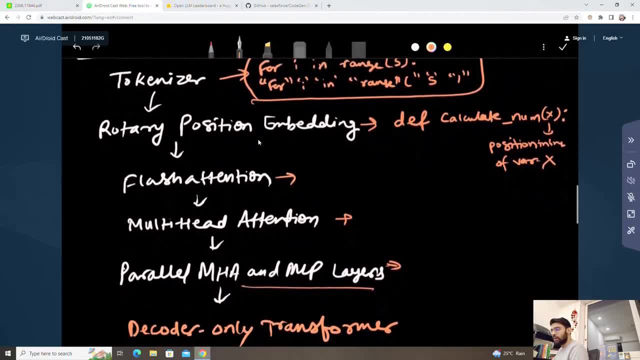 attention very quickly okay before moving to other guys here okay the multi-head and parallel image here so for let's take an example so flash attention so i'll take an example if 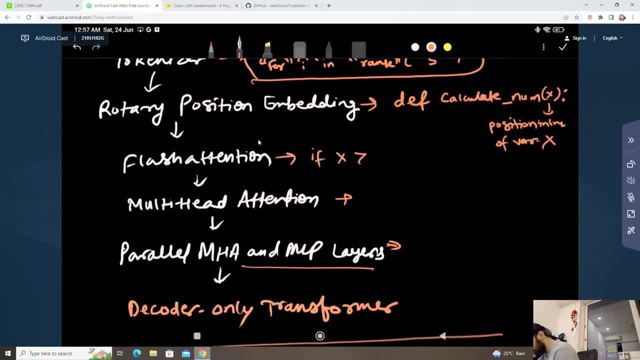 so if x greater than 10 if this is my code base okay if x greater than 10 put some result or 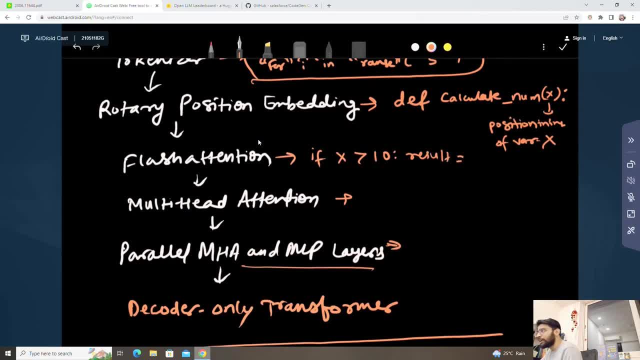 something okay now you have some result there can be you can just write x multiplied two or 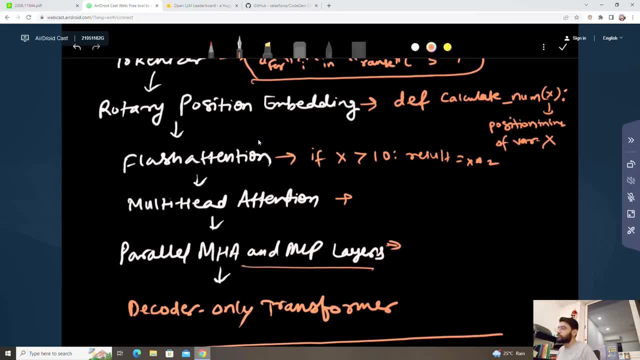 something so it model to focus on the uh uh comparison operator so we have this operator 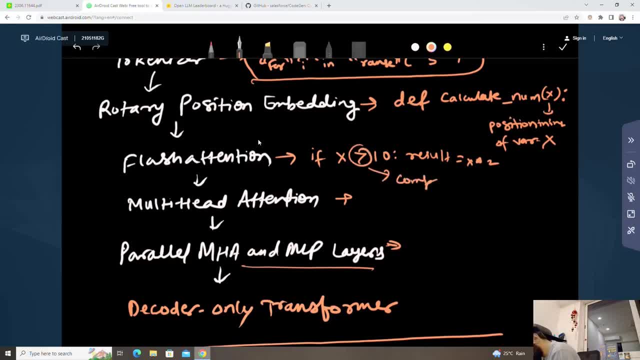 here okay this this comparison operator so basically flash attention what it does 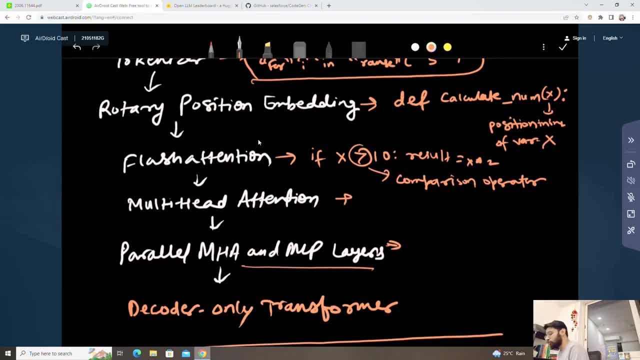 and the multiplication operation so whatever operation that we have so you see this multiplication operator so i'll just 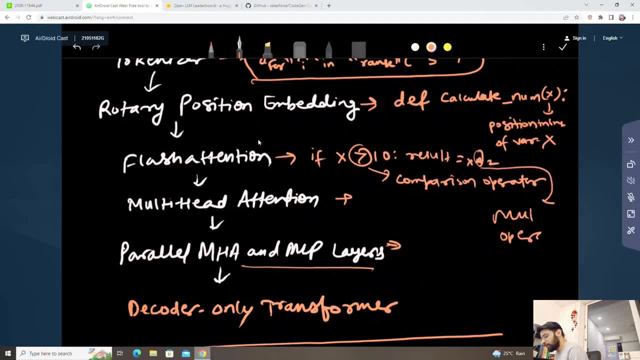 you just write multiplication operator and then we 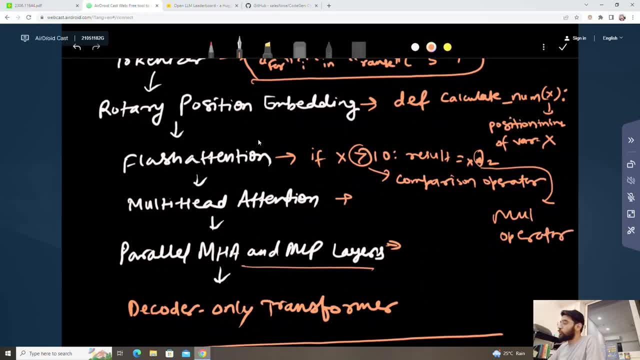 have comprison operator it focuses on this operation when predicting the next part of the code so it also predicts the next part 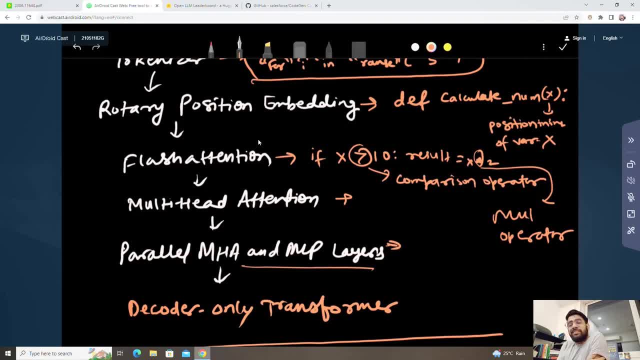 of the code album so it it specifically modifies the attention mechanism guys you know uh to improve efficiency and accuracy so mathematically it adjusts the weighting and importance of 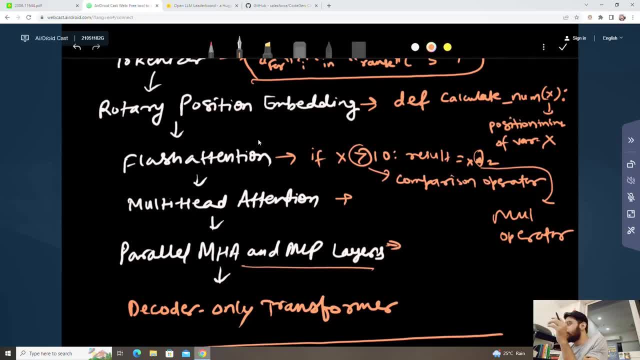 different tokens in the input that we are giving okay and enhancing the Goddess ability to focus on a specific code elements so like for example in this operator in this case 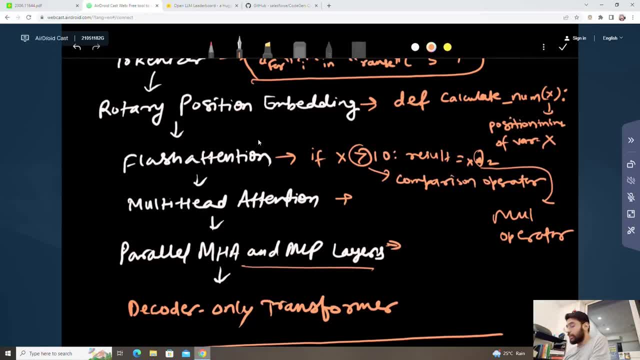 right it focuses on this and then it looks at what kind of sequence it can generate okay and then we have multi-head attention which now to 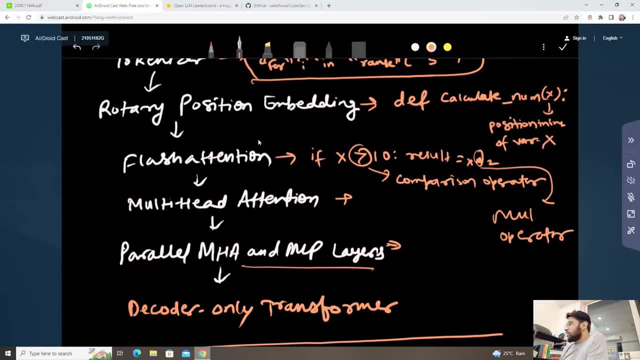 split into the multiple subspaces and i think it will get bigger guys so what i will do you know 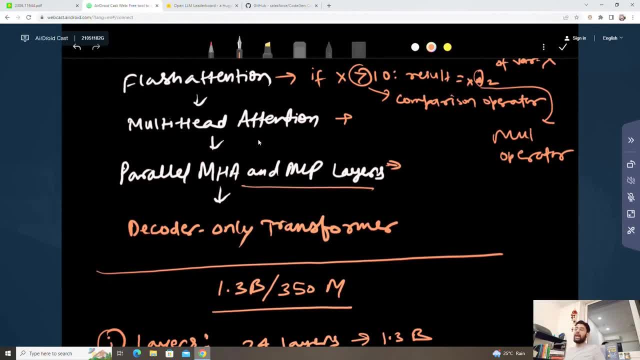 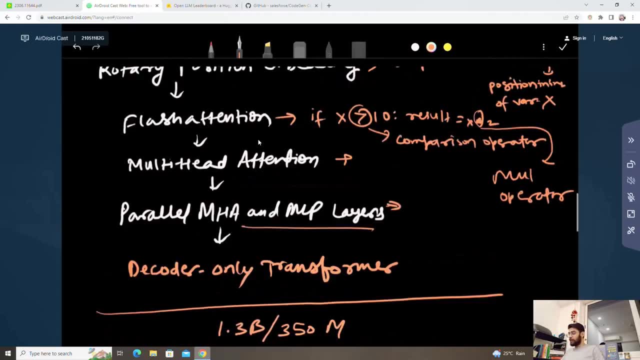 let me know your views on this because i don't want to go deep dive that technical of taking examples and talking about it so but these are the steps to organize the rotary 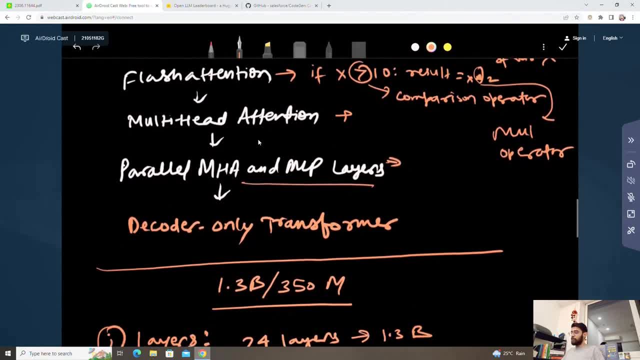 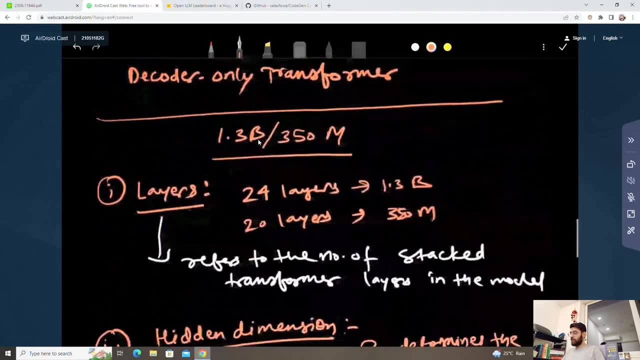 position embeddings flash attention multi-head attention parallel mha and mlp layers okay and and these are the hyper parameter that we discussed right layers